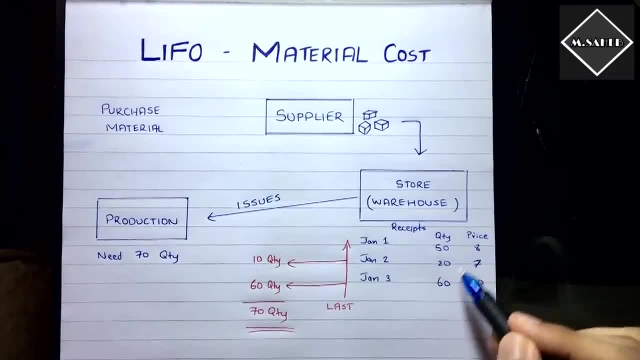 And on 3rd January, 60 quantity at the price 8.. Okay, so these much quantities you have in your warehouse right now, All right. and let's say your production department requested 70 quantity. So now the main thing is here: How are you going to send out this 70 quantity? Now you have to think from the point of your warehouse, because here in this LIFO topic, what do we do? is we prepare a stores ledger account? 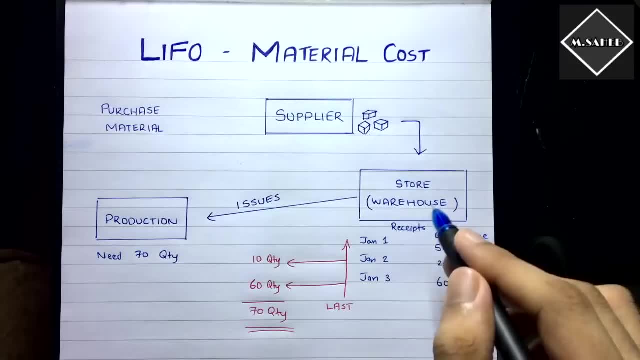 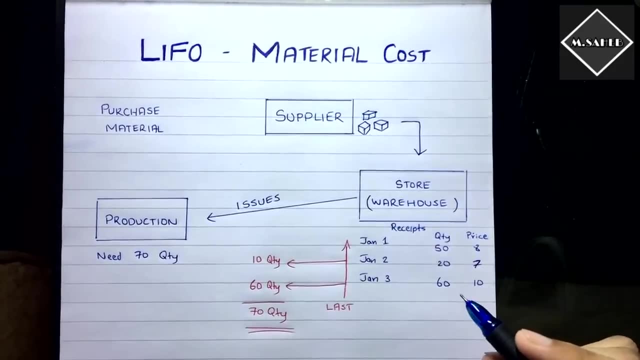 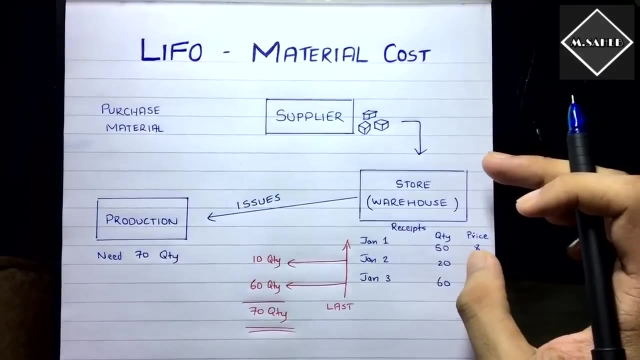 What A stores ledger account to keep track of all the raw materials that is there in the warehouse, Yeah, how the materials are coming in and how the materials are going to be sent out, The inventory. So it's very simple. See here: stores ledger account. There will be a receipt side- How much has come in issue side, How much has gone out, and then balance. 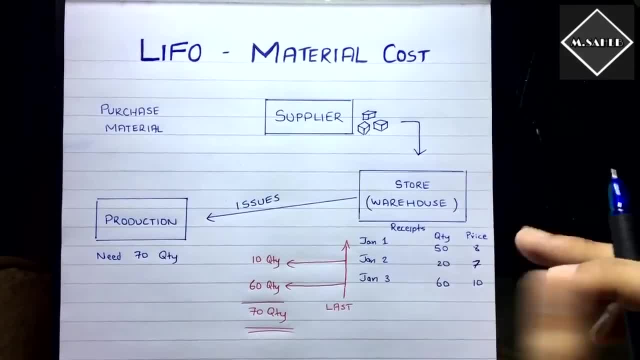 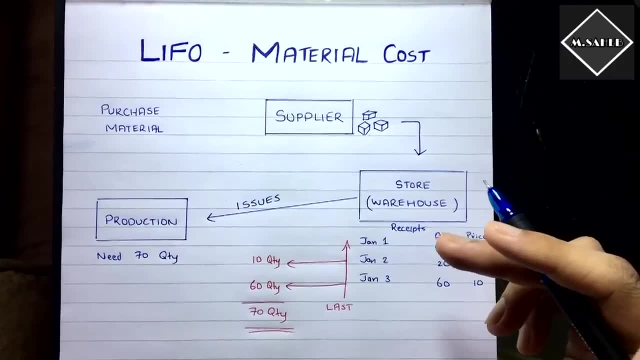 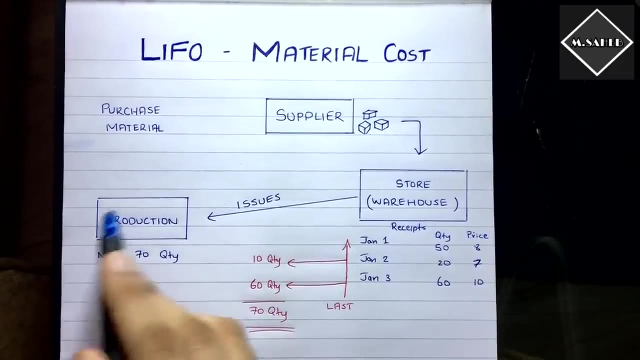 In balance. you are going to show what is there right now in the warehouse. Yeah, that is what is stores ledger account, and that stores ledger account is prepared on different different methods under different different methods. Yeah, FIFO, LIFO, AFCO. Yeah, simple average weighted average. So now see here What will be happening here. See here: in the production department they requested 70 quantity. 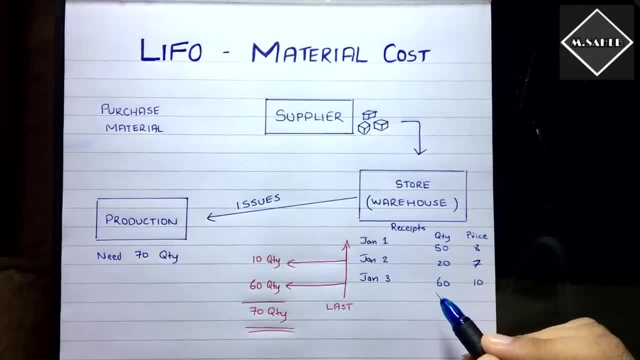 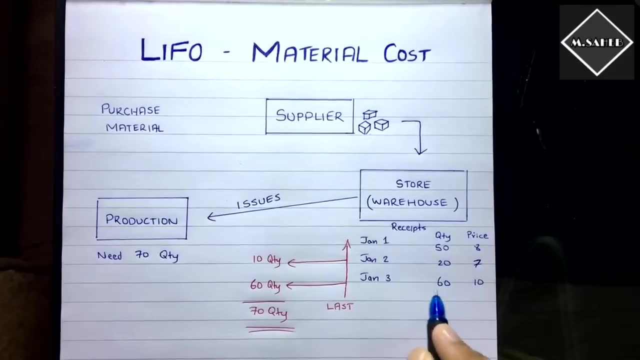 So under LIFO method. So under LIFO method, what you are going to do is to send out the 70 quantity. you have to follow a particular order. first, you are going to send out the 60 quantity at the price 10. okay, but that's not enough. they. 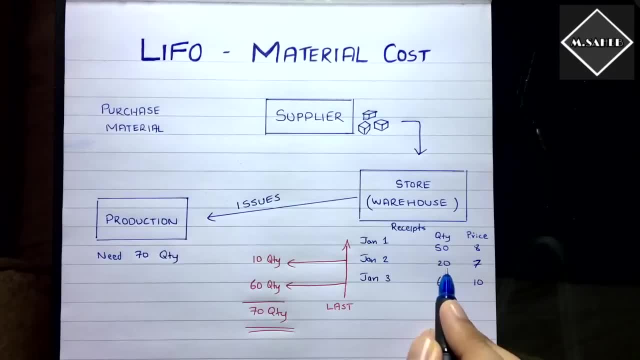 need 70 quantity. so what are you going to do? you are going to touch the latest, next lot, that is, second january lot. second january order: yeah, 20 at the price 7. so you are going to take 10 quantity from here at the price 7 and add it all up and you are going to send it to the production department. 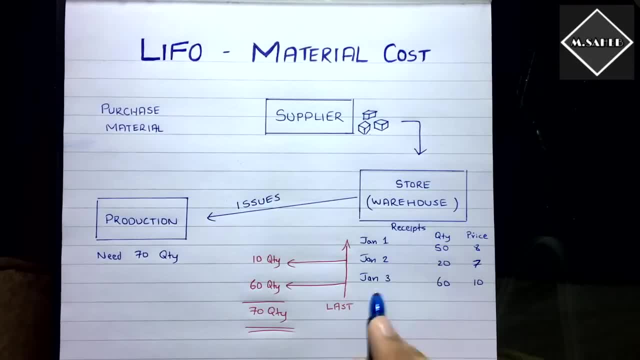 you see this last and first round, you have to touch the latest order first, and then it's not enough, then touch the next latest, next latest, like that. okay, it's exactly opposite to the fifo. in fifo we used to go, you know, first january, second january, third january. yes, here what third. 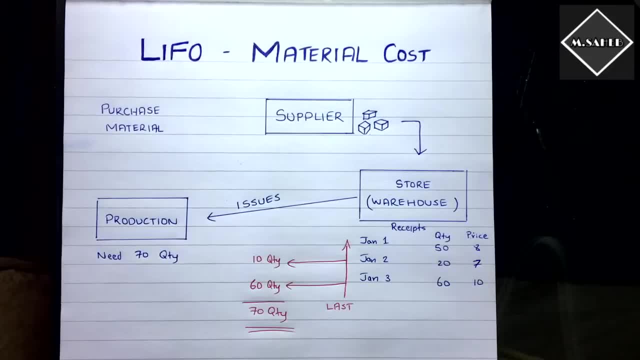 january, second january, first january, opposite. okay, and now you will be wondering: how does the valuation comes into the picture? here you are explaining that, the quantities. yeah, see, here we are not just taking the quantities, the prices also in the reverse order. yes, that is what is lifo method: valuation of inventory. and how are we? 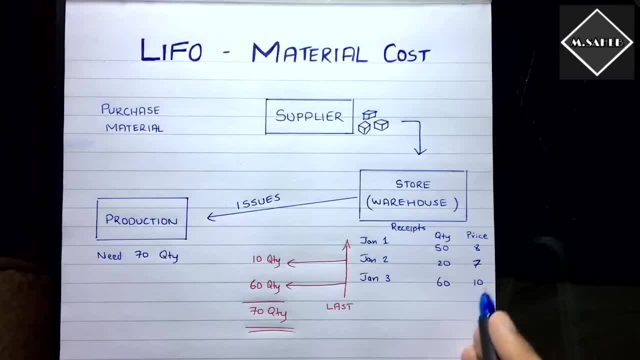 going to do that. we are going to do that by prices also. yeah, how are we taking prices? that is also very important. yeah, yes, so this is what will be happening. yeah, whatever that comes in last, it has to go out first. yeah, last in, first out. what is the last here? third january order, so that will. 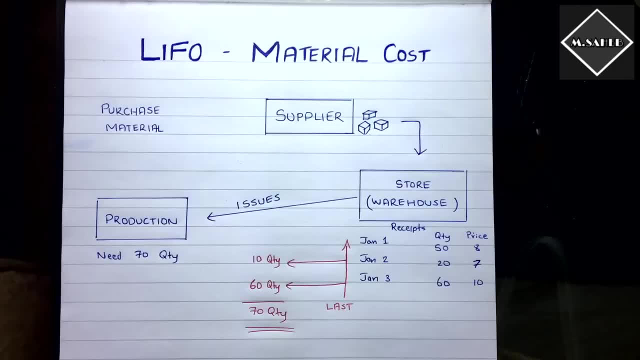 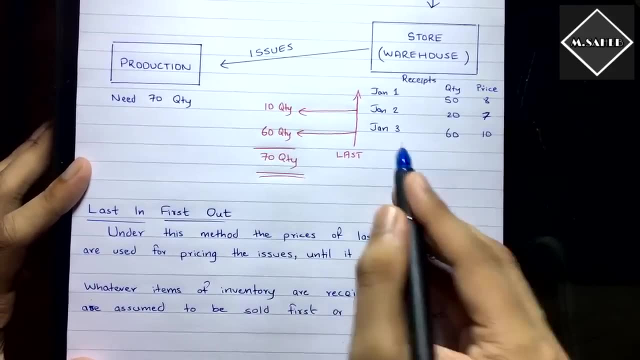 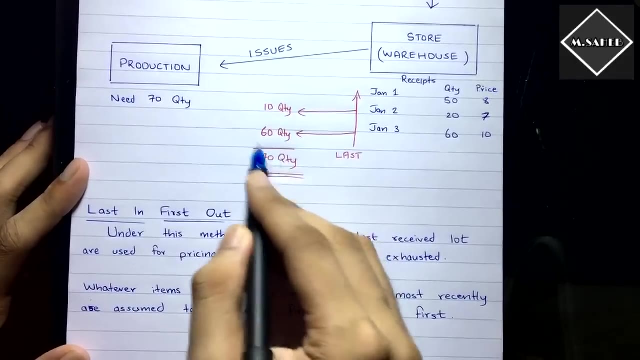 go out first and then second january, like that, exactly opposite to fifo. understood simple right. so see here, under this method, the prices of last received lot, the latest lot, third january, yes, are used for pricing the issues. yes, we are pricing. we have to price the 60 quantity, we have to value the 60 quantity. 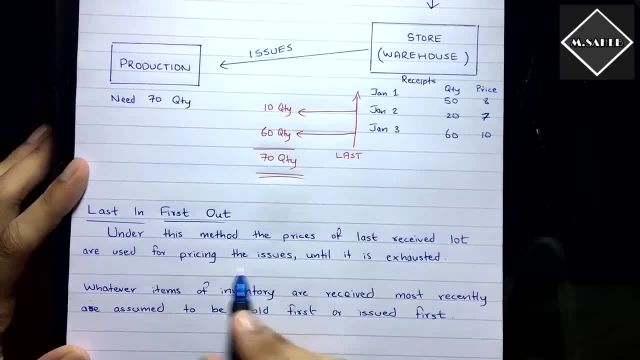 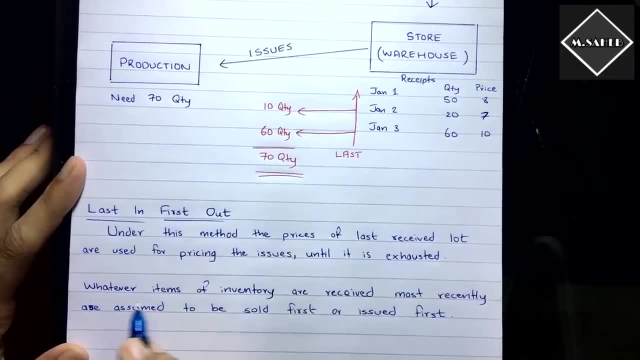 and which price we are using. the latest price rupees 10. yes, pricing the issues until it is exhausted. we have to go on doing that until it is. you know there is nothing left right. whatever items of inventory are received most recently third january, most recently- are assumed to be sold. 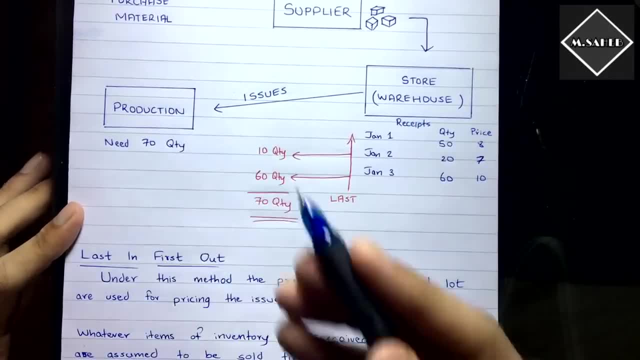 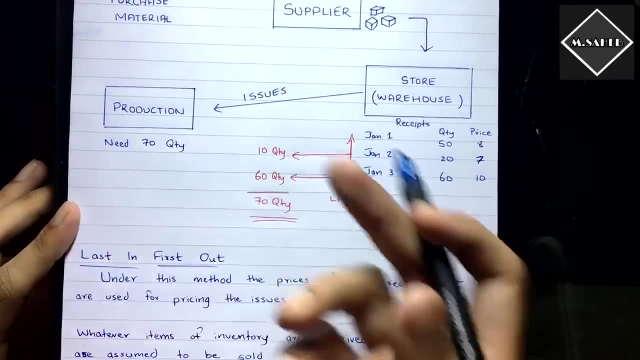 it is a production department, materials will be sent out to the production department and if it is, you know, a retail business, then what will be happening? from the warehouse, the materials, the inventory will be going out to the showroom to be sold. that is what is meant over here, or? 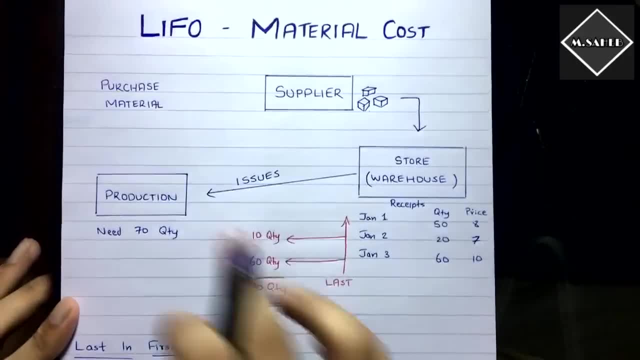 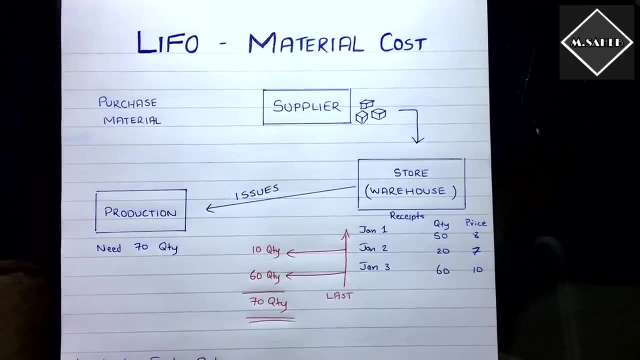 assumed to be sold first or issued for simple. whatever that has come in last has to go out first. now let's solve a life for practical problem and let's see how to prepare the stores ledger account. let's go to the problem now. here we have the problem. see the question over here. 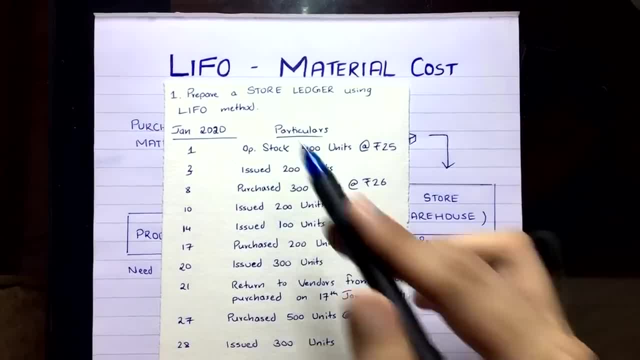 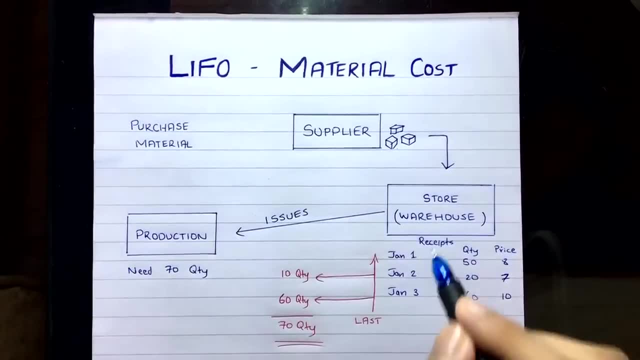 prepare a store ledger using life formatted. now we already know the price for a store ledger for summer delivery, so why do we have this topic? let's test this out. what is store ledgers? store ledger is an account that is prepared by the warehouse to keep the track of materials right: how much is coming in, how much is going out? 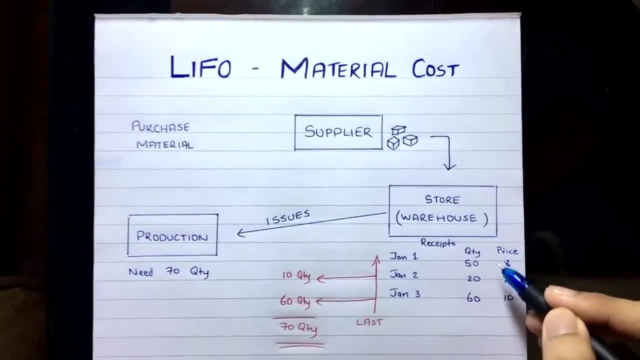 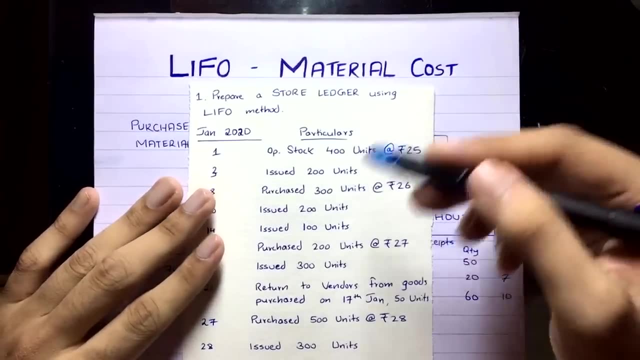 and how much is there right now in the warehouse. that is called balance. yes, so to keep the track of all this, yes, how much quantity is coming in and what prices it is coming in, yes, at what prices. so to keep the track of all this, an account is prepared. that is called store ledger. 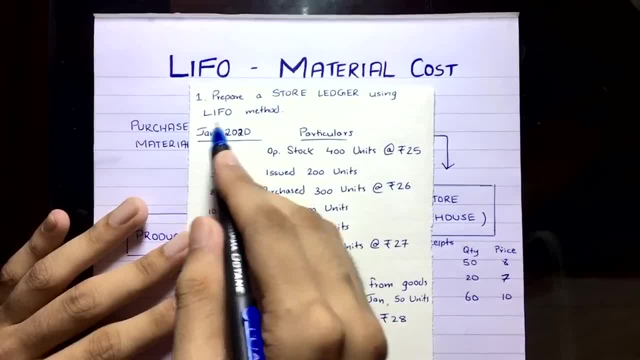 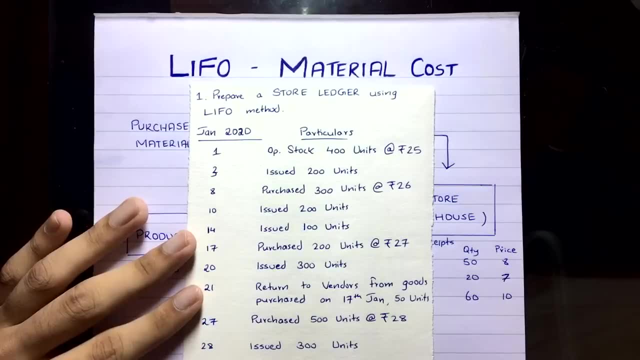 account, and that is what we do here in this topic. we always prepare store ledger, but under different. so this problem is of LIFO method. so store ledger will be prepared under LIFO method, understood, yes, so now here we have been given a lot of information. you 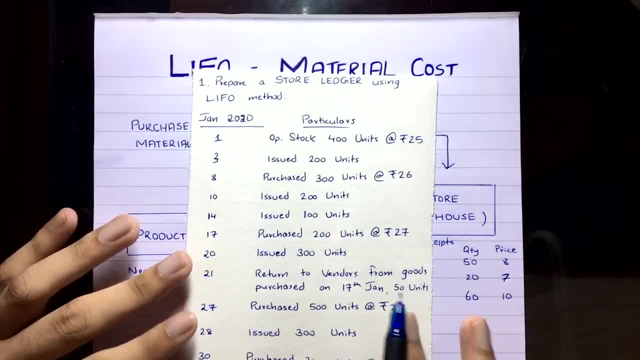 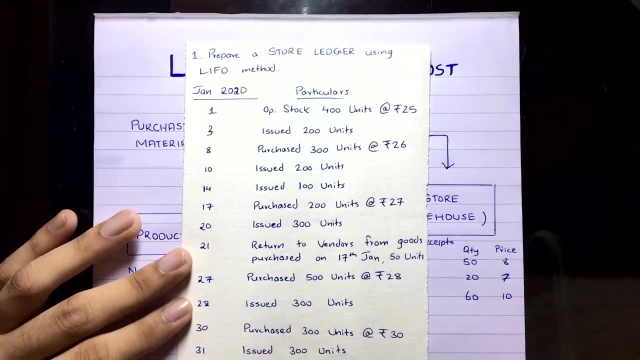 see opening stock. how much material is coming in, going out, yes. and then the interesting thing is see here: returns is given. yes, what is this? purchase return? purchase return is given. so we have to see that. okay, that's very interesting. and then, if you see here at last, on stock verification: on 31st January a. 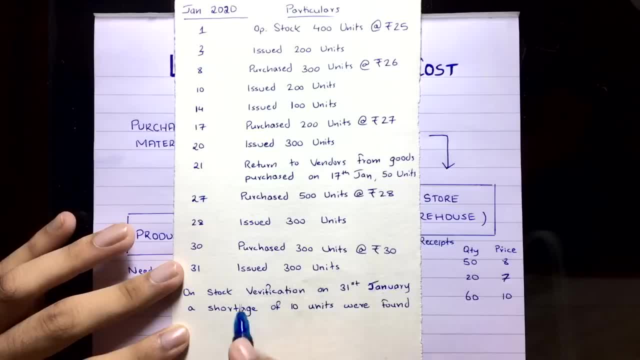 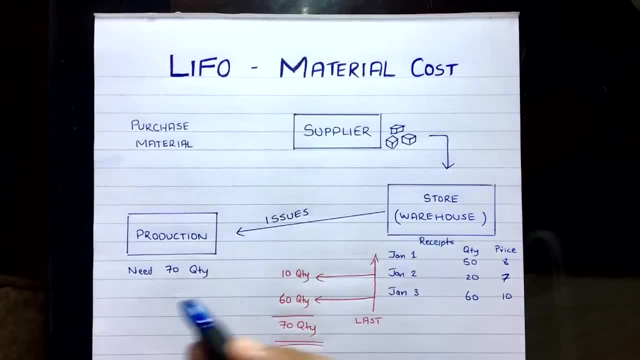 shortage of 10 units were found. so see this, this is what this is: abnormal loss. yeah, we have lost 10 units. so that means we have lost 10 unit means it has gone out of the warehouse. yeah, that is what we have to assume and we have to make an 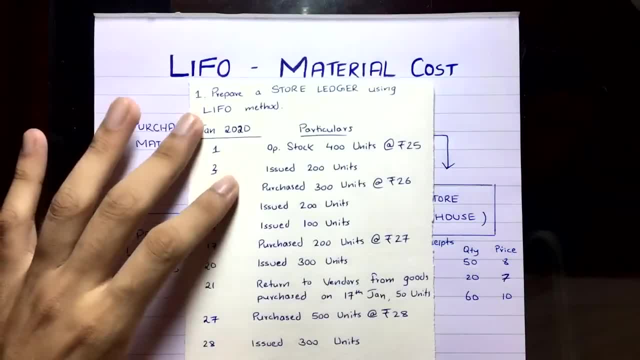 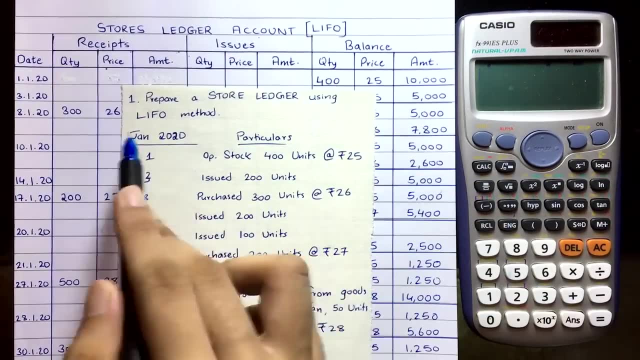 entry for that in the store ledger account. it's very simple. we will solve this problem now. okay, let's solve this problem now. let's solve the problem, yes, and let's see how to prepare the stores ledger account under LIFO method, as asked in the question. so the format of the stores ledger account will be the 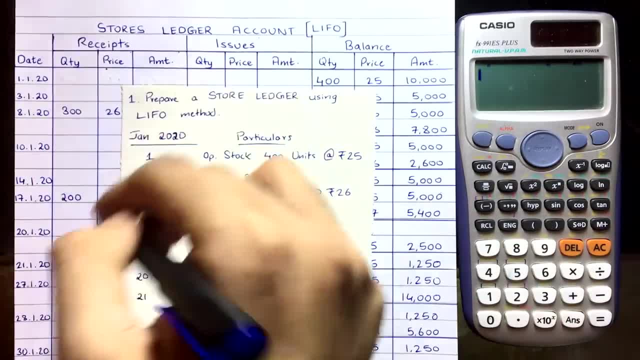 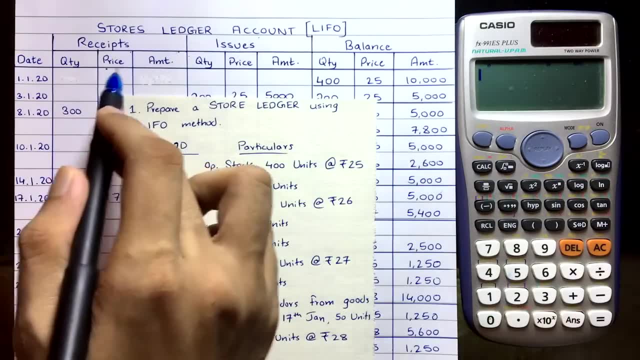 same format. yes, what we saw in the FIFO method: date column, receipt column, issues column and balance column. and then there are three sub columns in the receipt, issues and balance columns. see here: quantity price amount. quantity price amount. quantity price amount. simple format. yes, whatever that is coming in will come on the receipt side, whatever. 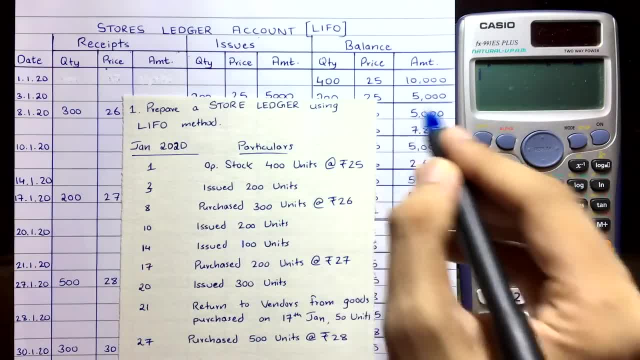 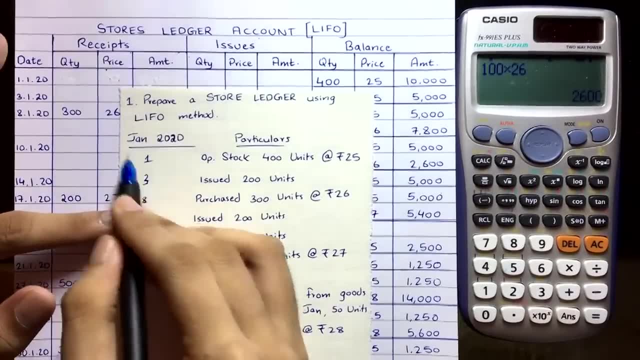 that is going out on the issue side and then what we have right now in the warehouse. that is the balance side. simple, that's the format you have to follow. okay, now the first transaction that we have got: see here on January 1st 2020. what has happened? we have got an opening stock of 400 units at 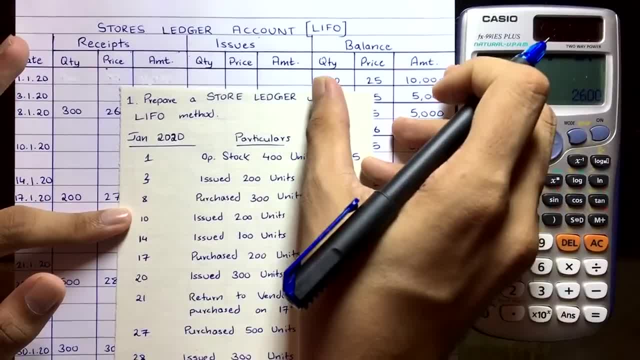 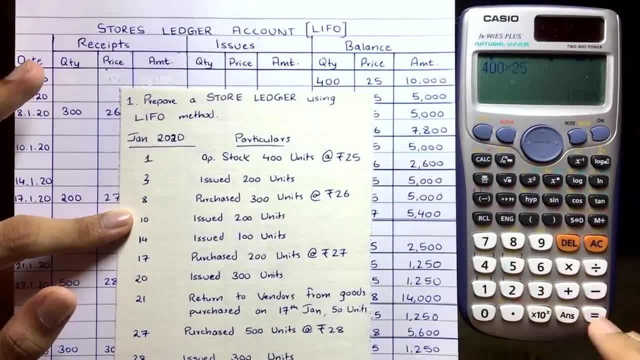 rupees 25. simple: opening stock will always go to the, directly to the balance side. simple: we have got 400 quantity at the price 25. so see here: 400 into 25, that is equal to 10,000. simple as that. yes, and then see on 3rd January what is. 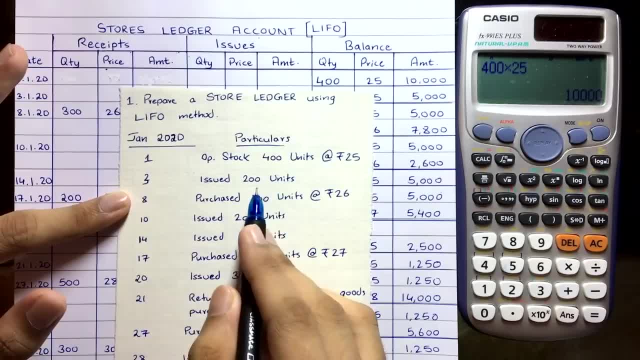 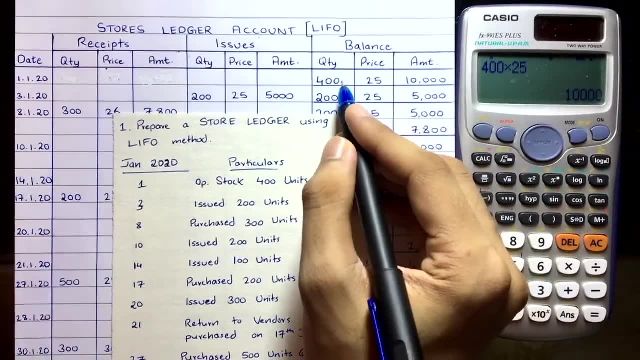 happening on 3rd January. we have issued 200 units. 200 units have to go out of the warehouse, so how will you send them out? simple from this 400, because there is only one Lord. yeah, here the life for the FIFO concept doesn't apply. yes, 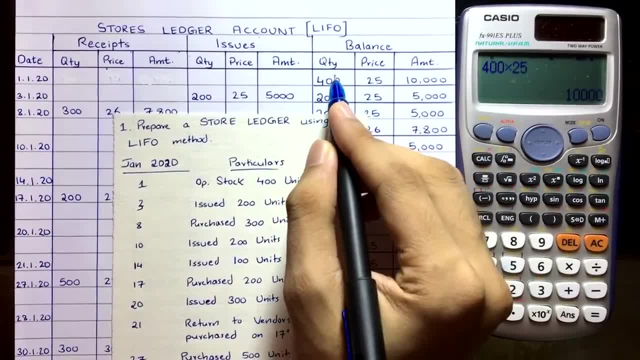 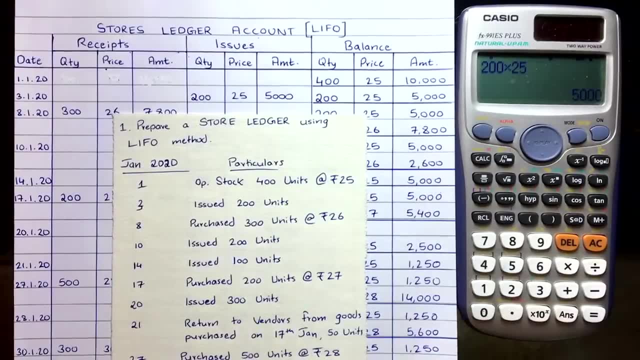 because there is only one Lord. so you have to pick from this lot only yes. so from here you have to take out 200, 200 at the price 25. so 200 into 25, that is equal to 5,000, simple yes. then what is remaining? 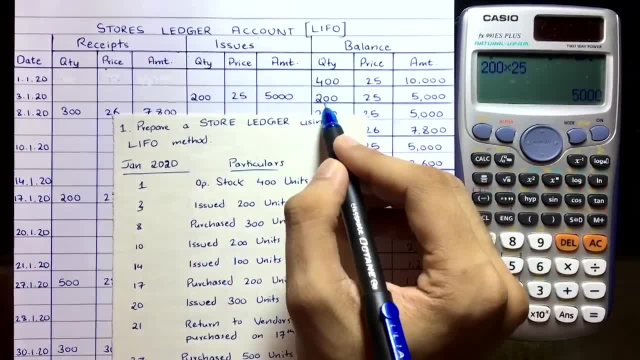 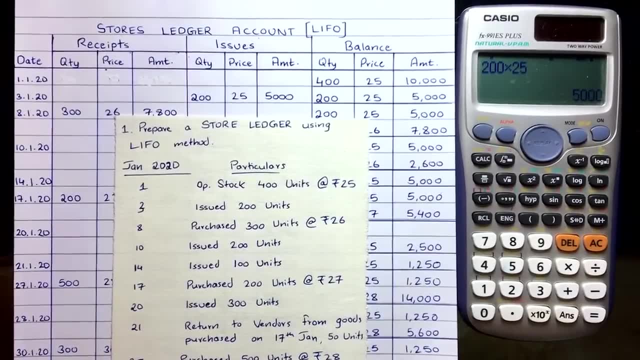 you had 400, you have sent out 200. remaining is 200 at the price 25. yes, so same thing here. 200 into 25, that is equal to 5,000, simple right. and then let's see, on the 8th January, what has happened. on the 8th January, we have 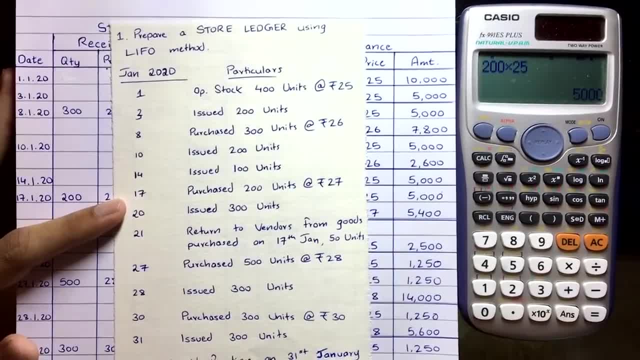 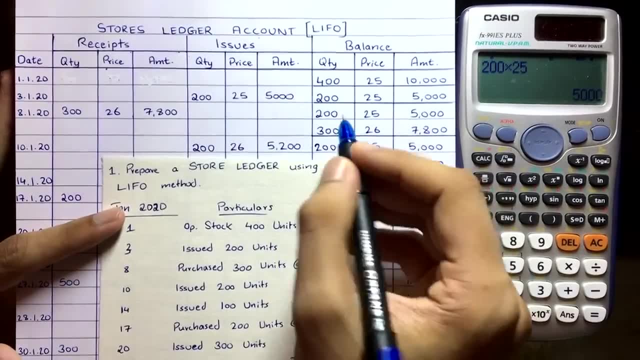 purchased 300 units at the price rupees 26. so now, in the previous video I've also told you, whenever we get a purchase, what we have to do. we have to do that right. what draw a line in the balance column? yes, and whatever that is there in. 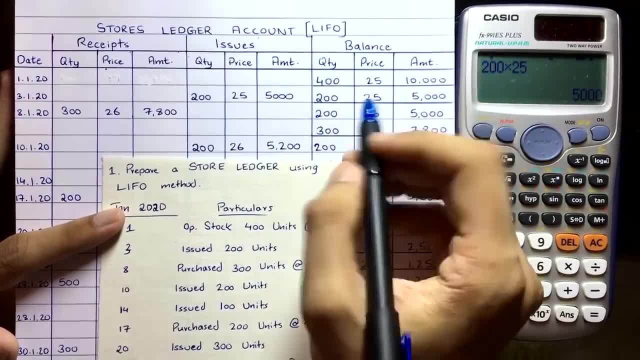 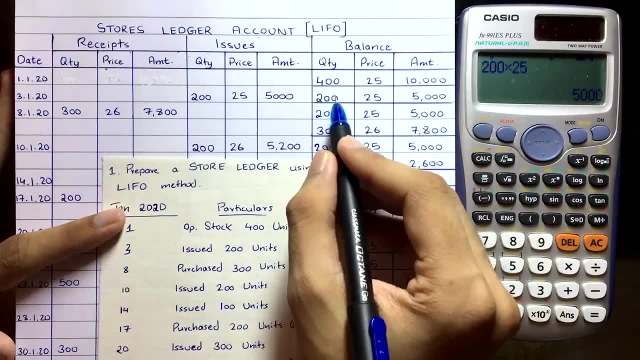 the balance column previously. we take it down: exactly 225, five thousand was there, yes, and then on eighth January, what happened? purchased happen. so now what we have to do, copy this, whatever that was there in the balance column down, exactly 225, 5,000, same. and then, whatever purchase you have made, take it and copy the purchase. 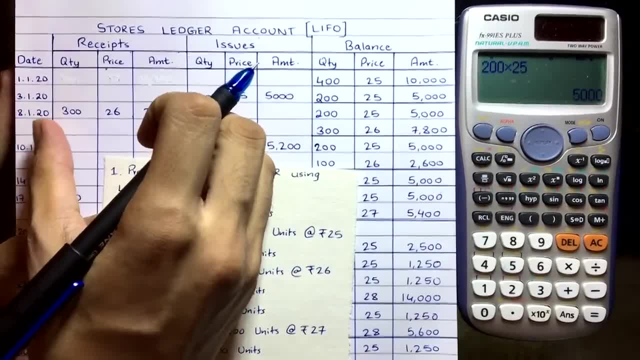 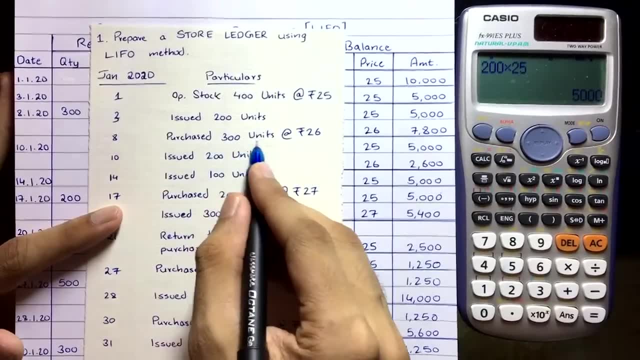 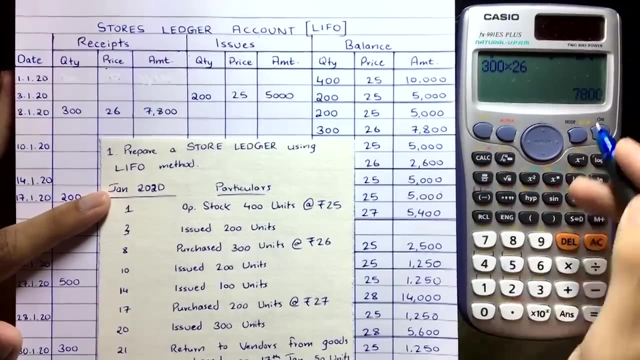 now we have obtained that, and then something has newly been called for, and then we have to deny another difference in the output, and then could be a that below this. yes, see here how much did we purchase? purchase 300 units at rupees 26. yes, so 300, 26, 300 at the price, 26, that is equal to 7800. so now you have. 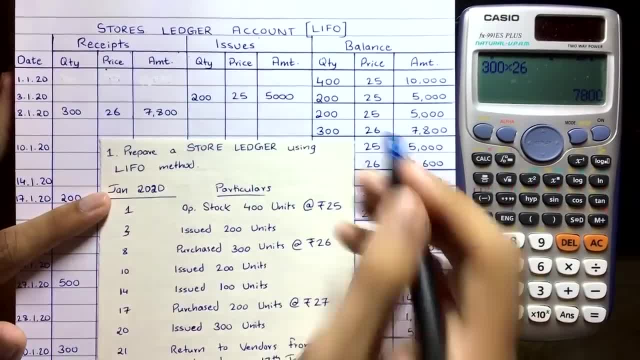 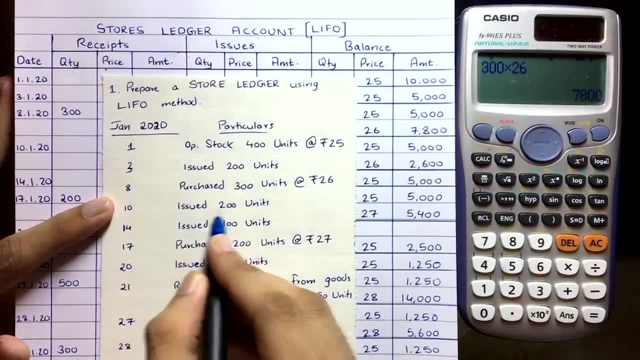 to take this and write it exactly below: copy paste, simple, you understood. yes, now let's move on. you will get that, okay, see here, on 10th January, what has happened then we have to issue 200 units. yes, how much 200 units we have to send out from. 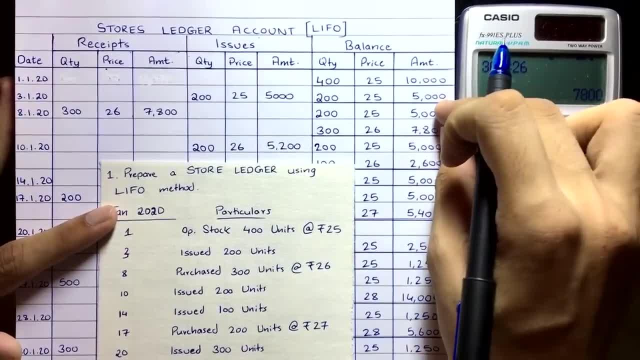 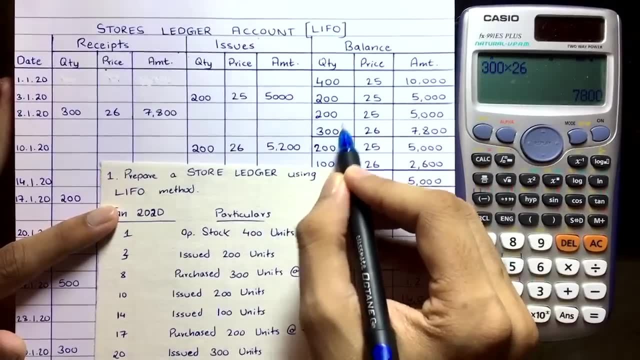 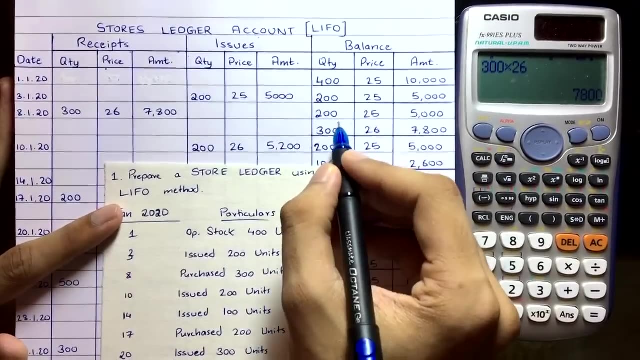 the warehouse. now how will you do that? in the warehouse you have these two lots now. yes, the old lot and the latest lot. we have purchased this one. yeah, so two lots you have now here. you have to be very careful. you have to see whether in the question they have said life for or FIFO, because here only the. 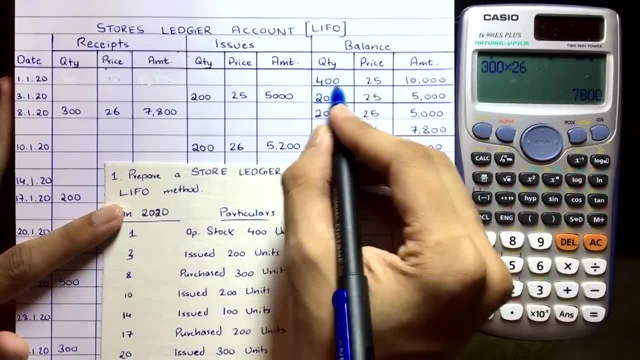 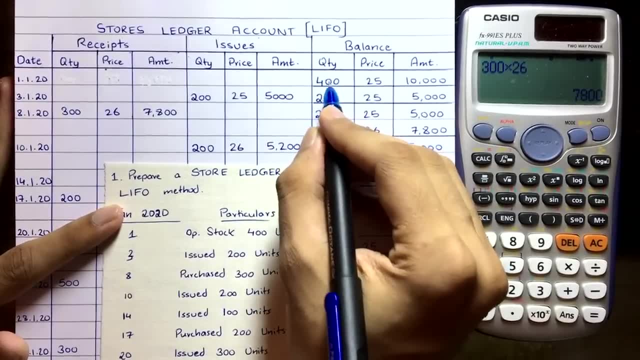 life for FIFO concept applies right, because here in the previously, if you see the first transaction, there was only one lot. so, whether it was like for FIFO, you have to send out units from this Lord, only one Lord, right, you have to to send it out from here, only 200, yes, but here now there are two lot. so you have to see whether 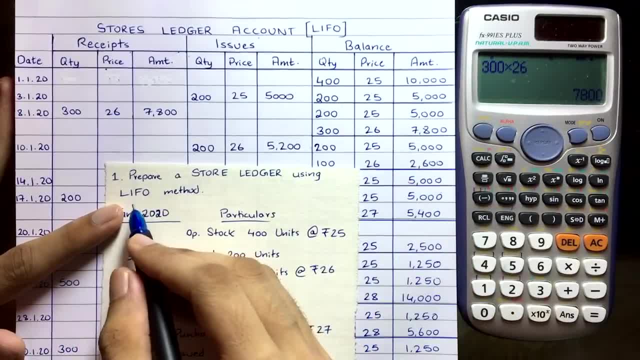 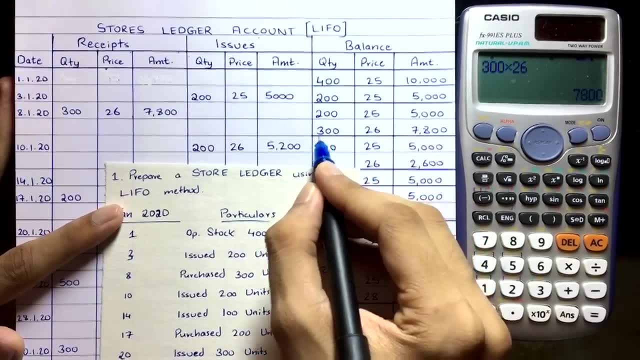 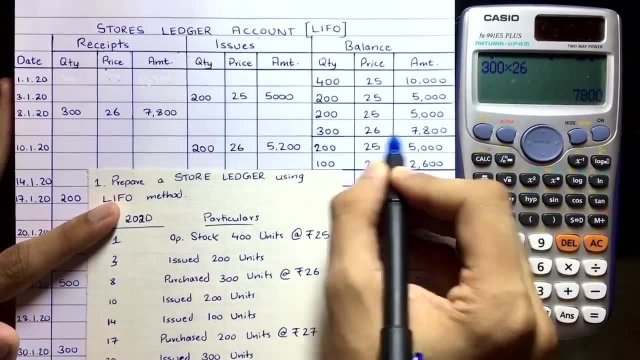 it is life or fifo, and do it properly, since this is life, for last in, first out. so what you are going to do, you are going to take the last lot and send it out first. yes, opposite of fifo, isn't it? so you have to send out how much? 200 units. so you have to do that from the last lot, latest lot, most. 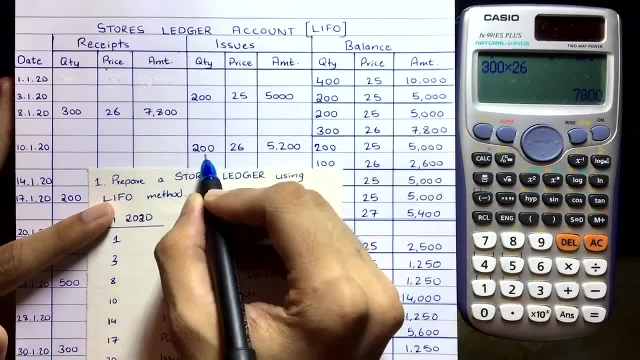 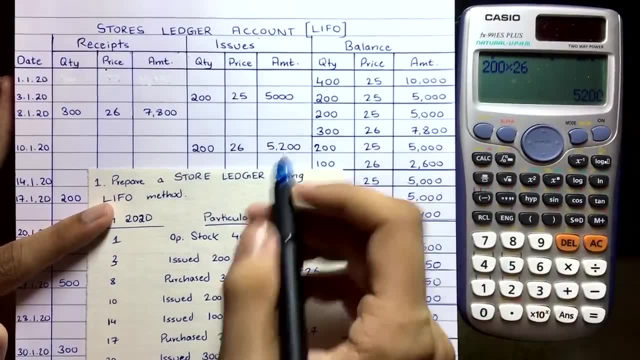 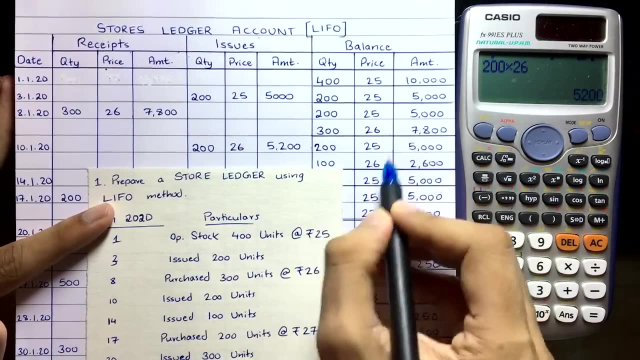 recently purchased lot that is 300. so from this 300, you are going to send out 200 and you are going to take that price only. yes, 26. so 200 into 26, that is equal to 5200. yes, understood. so this much you have sent out. now, what is remaining in the warehouse? yeah, that you have to write here. 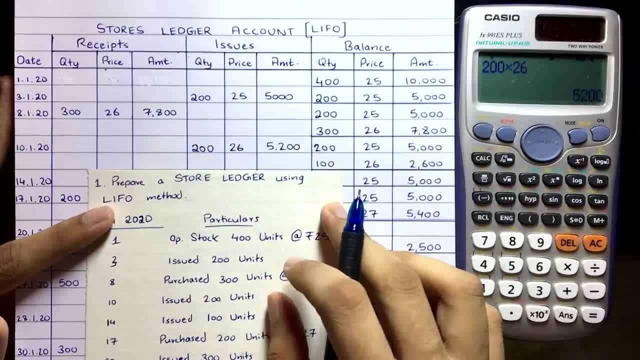 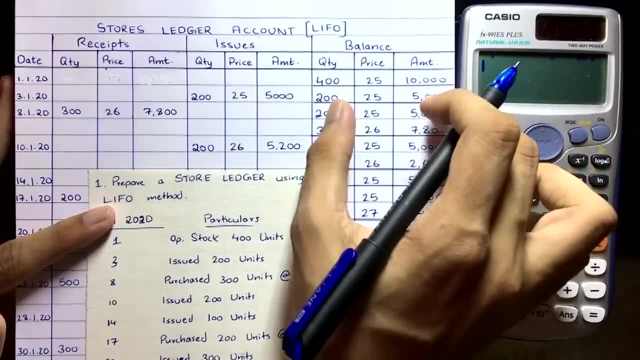 on the balance side. simple, right next to that, okay, simple. so see here what you are going to do. you haven't touched this first lot, right, you haven't touched this first lot, so what are you going to do? you are going to take the exactly, it is remaining in the warehouse, right? so you have. 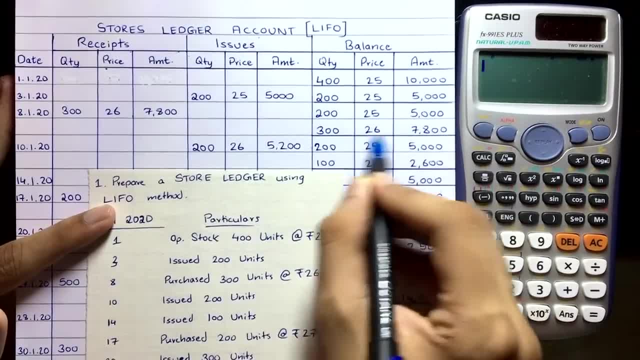 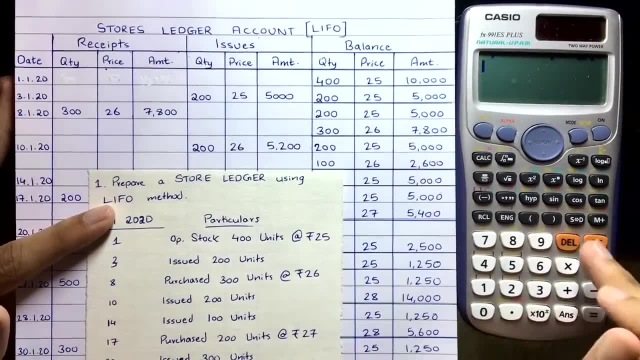 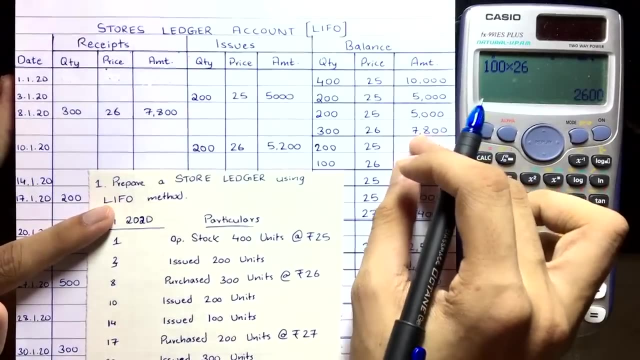 to write that down. and then you have touched only the latest lot, yes, this 300 quantity lot. so now, if you have sent 200 out from that 300, then the remaining is 100. so 100 into 26, that is equal to 2600, simple. so now these two lots are remaining in the warehouse. 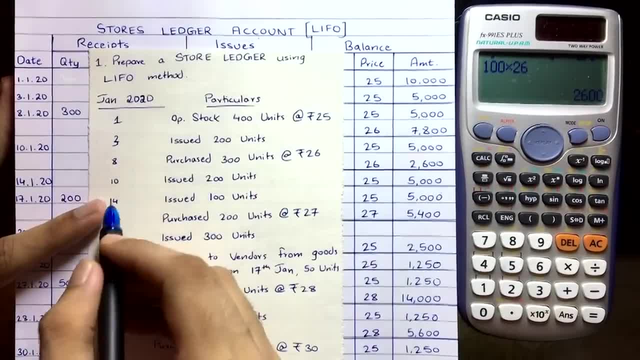 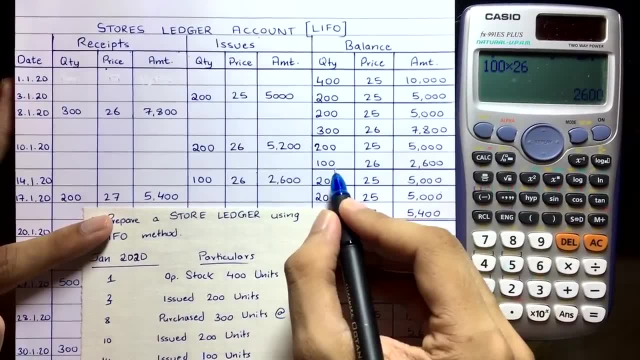 simple as that. okay, then let's move on. let's see then on 14 january, what happened on 14 january we have issued 100 units. okay, issue 100 units. so now what you are going to do, which lot- this one or this one, the latest, the last lot? this one: 100 units. so now what you are going to do, which lot. 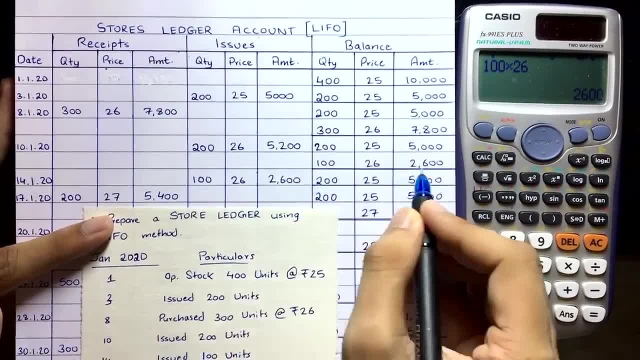 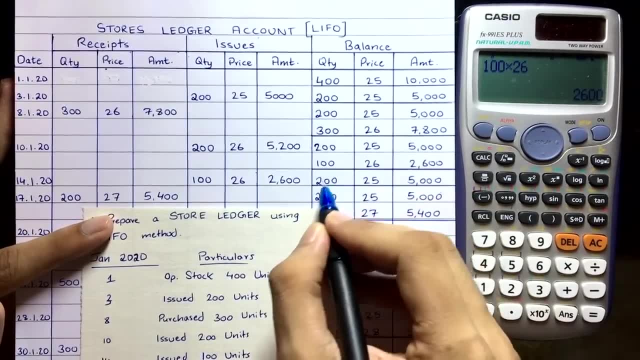 is this 100? yes, so send it out: 100, 26, 2600, the same thing, yeah, entire thing. you are sending out. then what is left? this lot is left. yes, yes, 225, 5000, simple, okay, then draw a line. yeah, then see what. 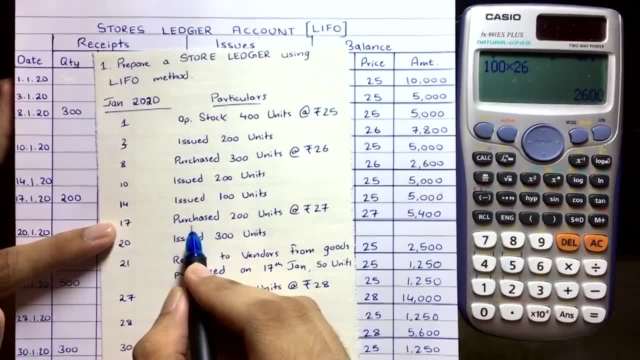 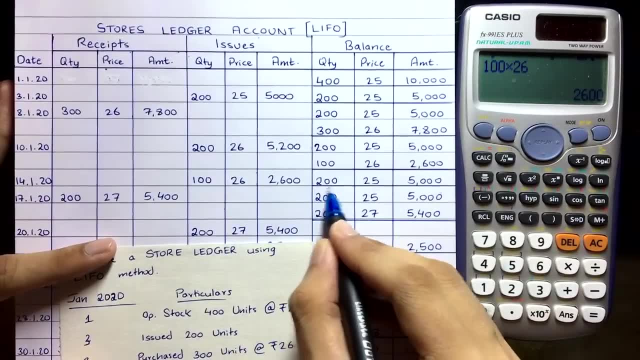 has happened on 17 january. what is happening? purchase. now again, whenever there is a purchase, what you have to do draw a line in the balance column. yes, here, right. so draw a line in the column. whatever that is there in the balance column. now, what do we have? 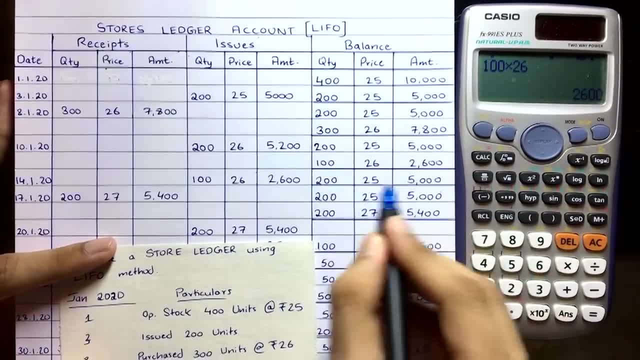 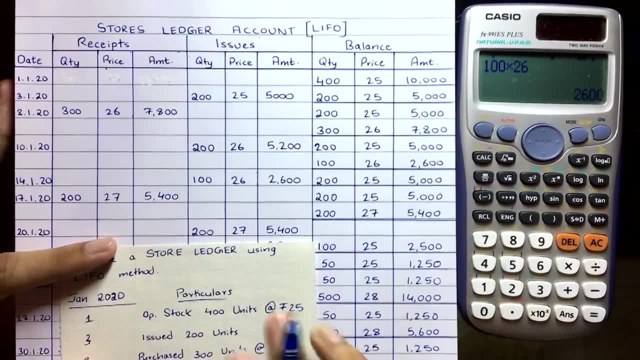 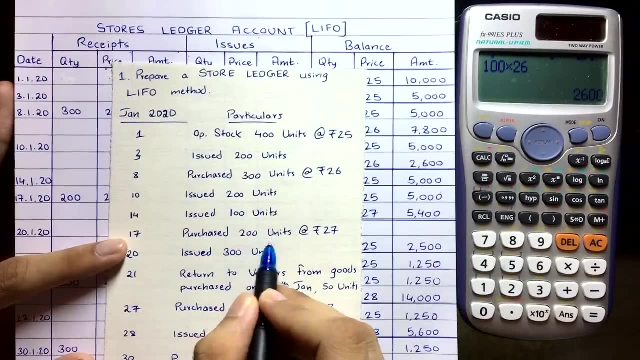 balance column 225 and 5000, isn't it? this is what is left in the balance in our warehouse. so copy that down exactly below 225- 5000 and then see what purchase you have made. see on how much: on 17th, right on 17 january, we have purchased 200 units at rupees 27. so 200 at price 27, that is equal to. 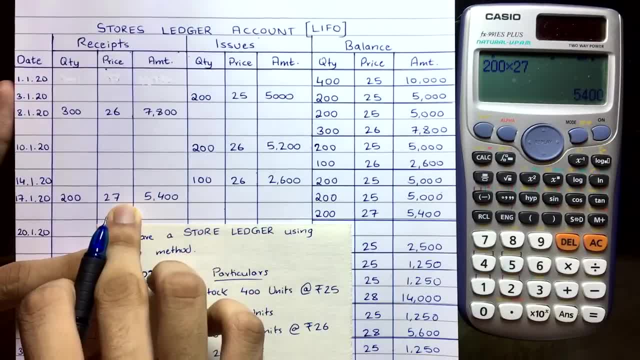 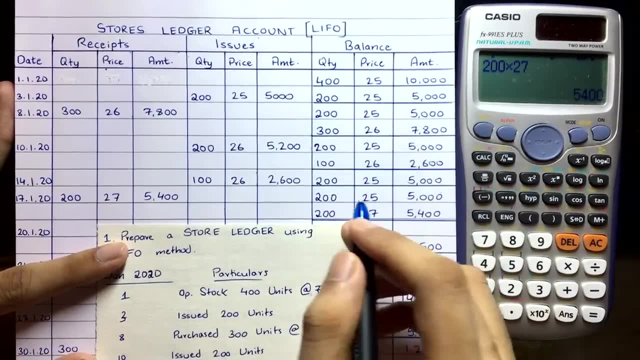 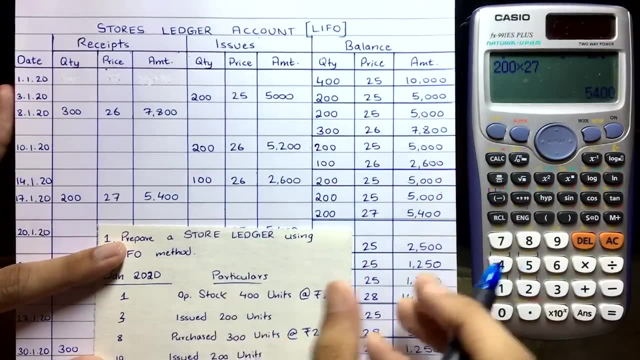 5400. take it in the receipt column, since you are getting it in your warehouse. yeah, 227, 5400. copy that and paste it exactly below that. yes, exactly below. in the balance column: yes, draw a line. take whatever that is there in the balance column below and then whatever purchase you have. 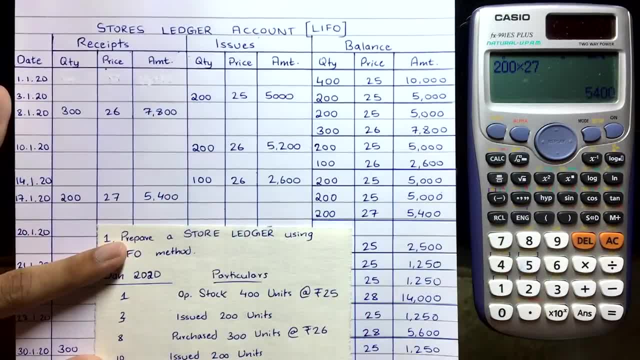 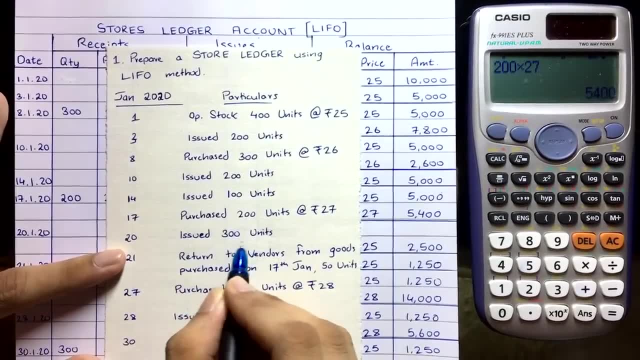 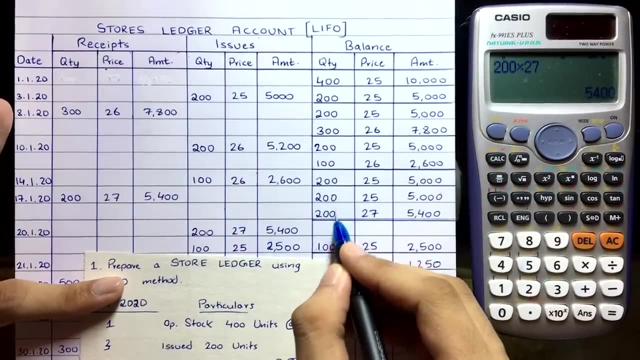 made. you have to take it exactly below that simple yes. and then what has happened on 20th january? on 20th january, see, we have to issue 300 units. how much 300 units we have to send out. okay, fine, so see here. now what do we have in the warehouse? 200, 200. 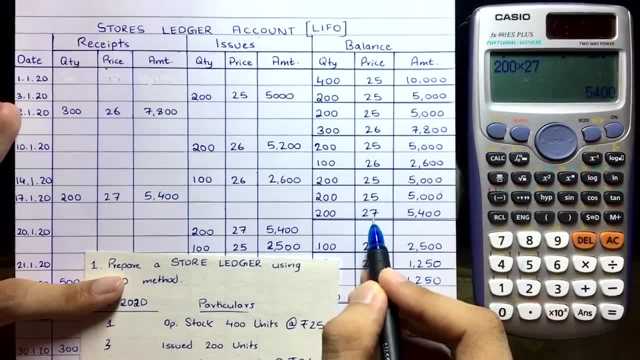 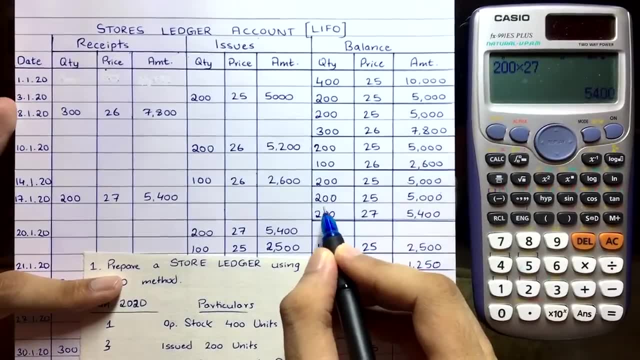 two lots we have. one is 25 price and the other is 27 price. fine, so see, here we have to send out 300 units and we have to follow life or right. last in, first out. so we have to do opposite of 5o. so first we are going to touch the latest lot. this is the latest lot, right, the last lot. 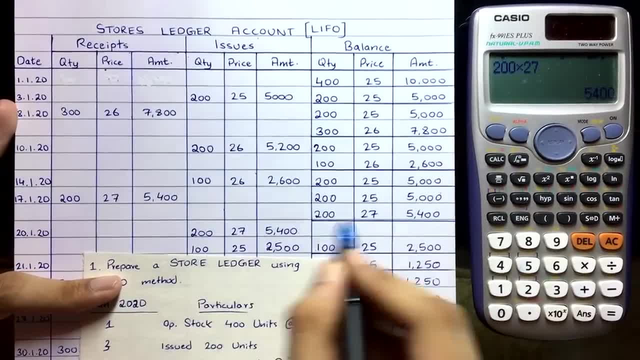 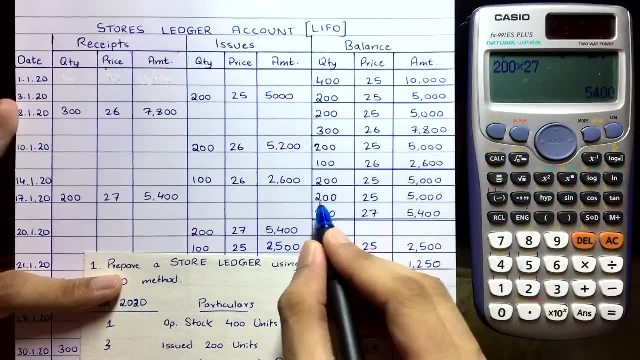 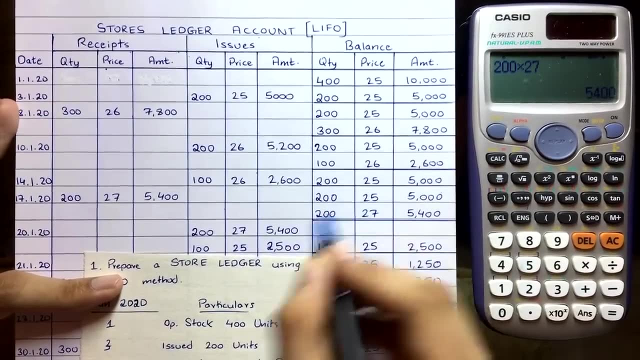 yes, 200. so first we are going to send this out 227, 5400, simple, and then, since we need to send out 300, so the remaining 100 has to come out of the next latest lot. so we have to send out that is this one. yes, yes, so you have to take 100 from this lot at the price 25. yes, so 100 into 25. 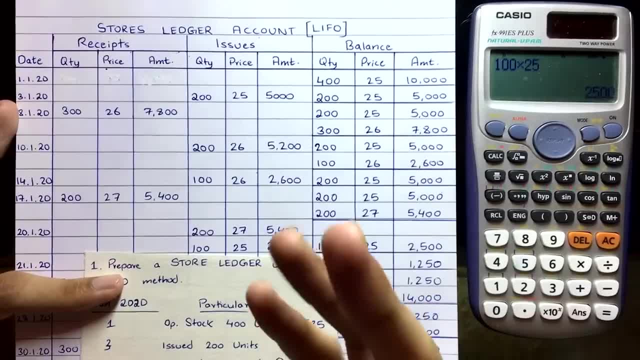 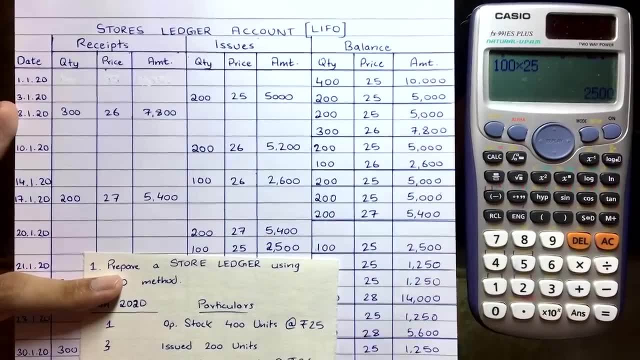 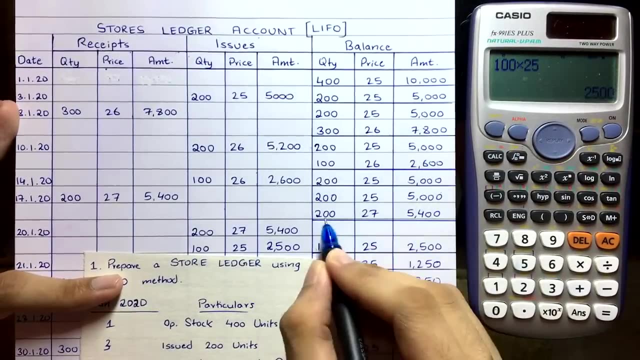 that is equal to 2500. you get this. you had to send out 300. first you touch this one, the latest one, and then you went back. yes, that was this one, simple yes. so this is what you have to do, and then the remaining you have to write it over here. okay, so now this one is entirely gone. 227 5400. 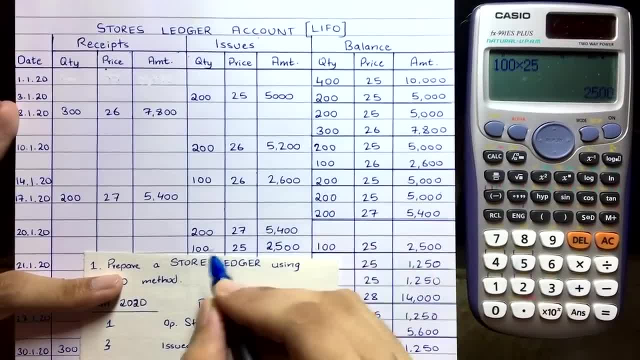 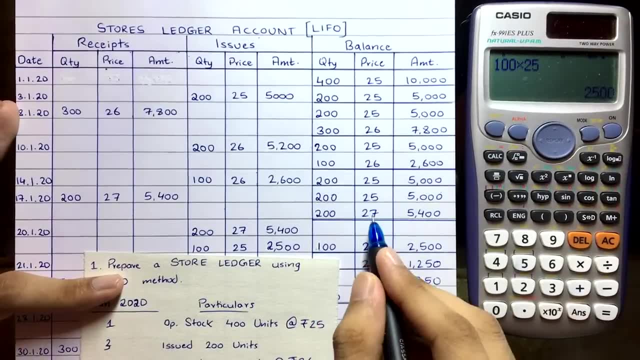 but this one is left right here. you have to write it over here, okay, so now this one is entirely gone. here you have sent out 100 out of 200, so here 100 is remaining, so that will come out over here. 125. this 27th one is completely gone. okay, don't take that. okay, you can take it, nil, but it's not. 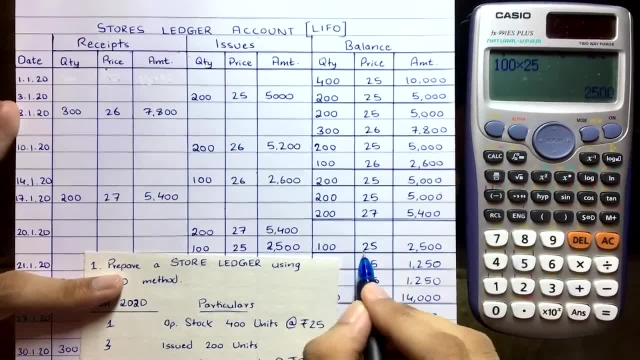 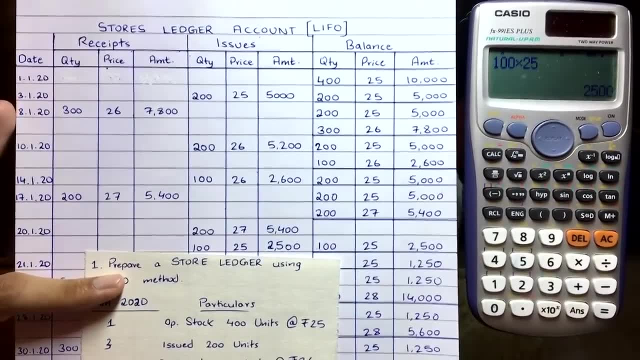 required. don't take nil also. okay, just leave that. and then 125, 2500. understood, because that is what is left right. 100 into 25, 2500. you understand that right? it's very simple, okay, then on 21 january, see here: return to vendors from goods purchased. 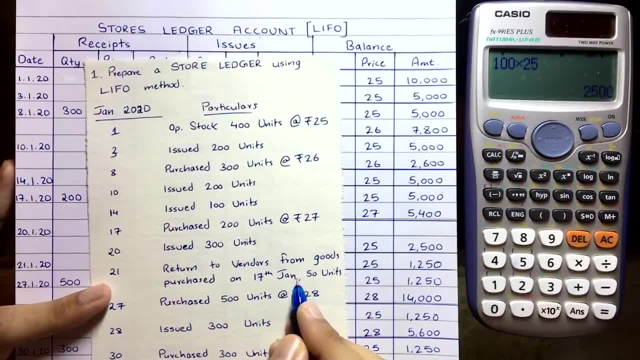 on 17 january? yes, 17 january, 50 units. what has happened over here? we have returned the goods that were purchased on 70th january. and what is the quantity of return? 50 units. it's not a problem, it's very simple. see here: what have we done is whatever that was purchased on 17 january, yes, at. 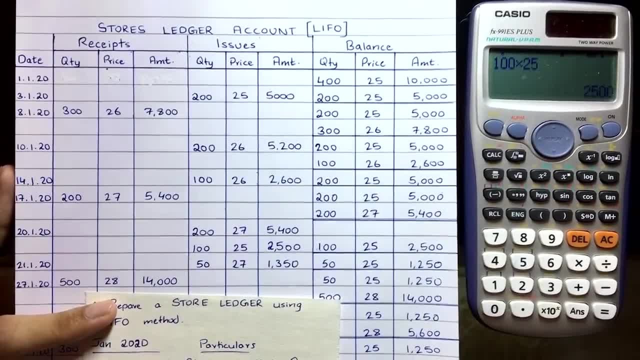 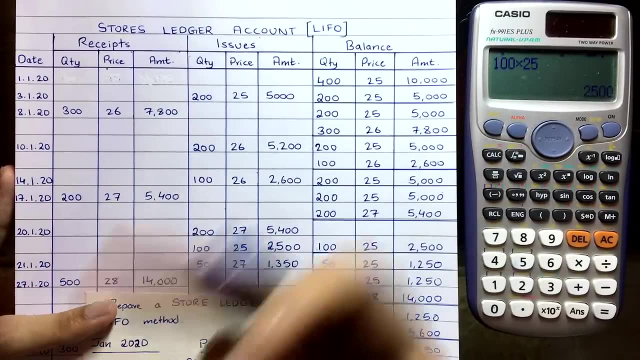 the price: 27, we have returned 50 units. how much 50 units? so simple return means what it is going out of our warehouse. yes, it is not sales return, it is purchase return. purchase return means what we purchased before, what was came in before. now we are returning it. it is going out if it was sales. 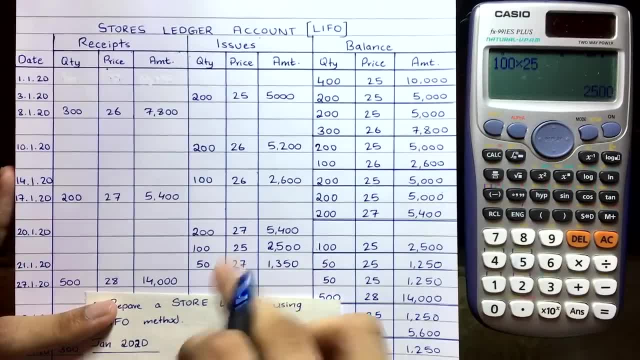 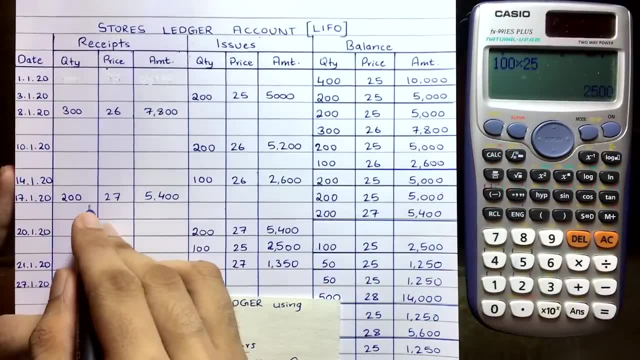 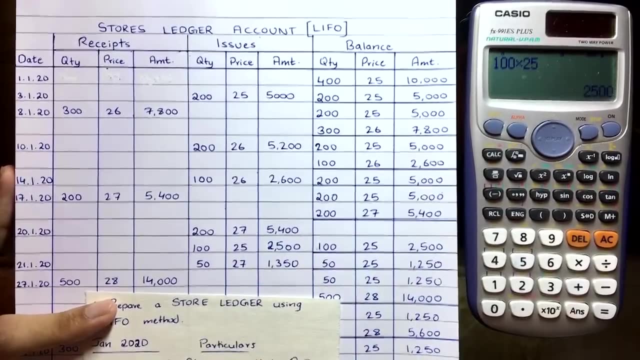 return, then what we have, you know, sold or sent out of the warehouse, it is coming back in. then that was purchased. i mean that was receipt, yes, but now here, what was purchased on 70th january, it is being returned, it is going out of the warehouse. so now you have to take that into issue. column simple. 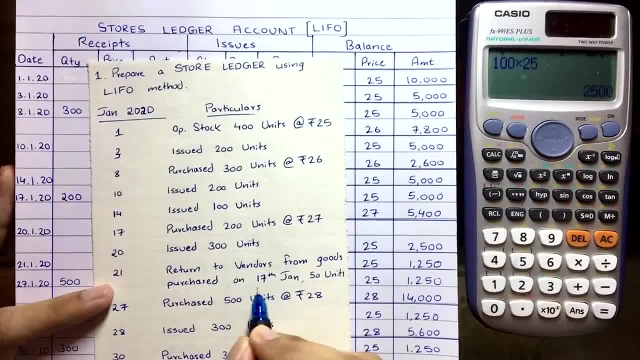 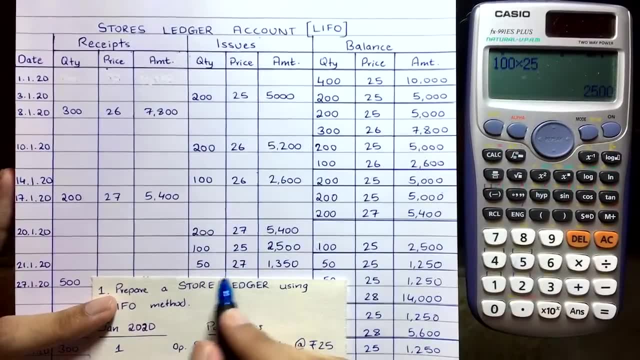 now, why did they give 70th january? because you have to use the price of 70th january. so now you have to use the price of 70th january. okay, so this price you are going to use 27, simple, you are going. 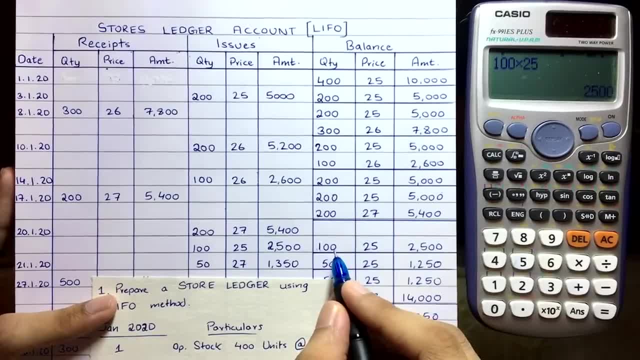 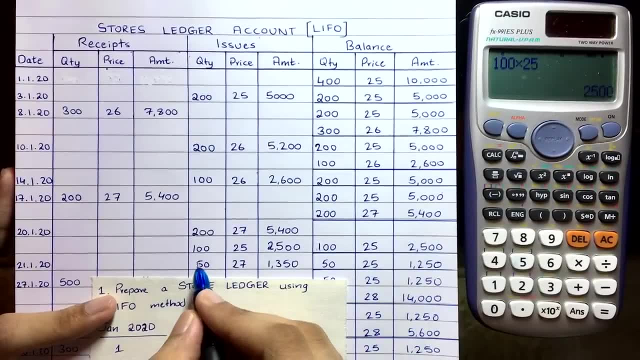 to send out 50 units. right now in your warehouse you have 100 units, isn't it so? 100 at the price 25, 2500, you have to send out 50.. simple, you are returning it. it is what purchase return. purchase return will always come here. sales return will always come here. okay, so see here 50 quantity. 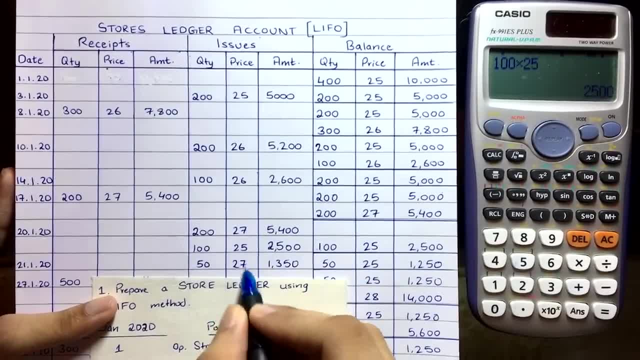 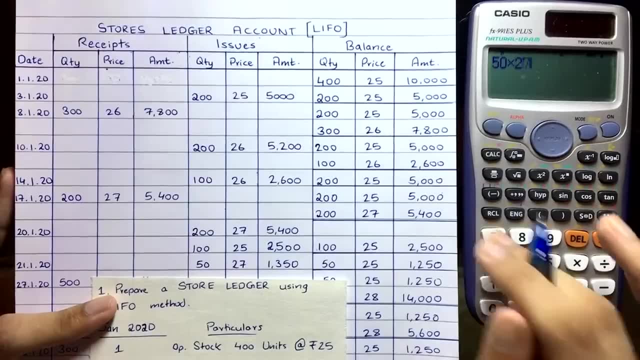 which price you are going to take, not this price, the price which was there on the 17th january, simple right 27.. so 50 into 27, that is equal to 1350, right, 1350. simple. then what is remaining 50 quantity is: 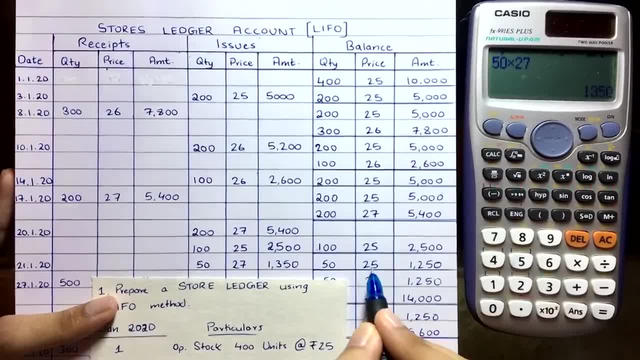 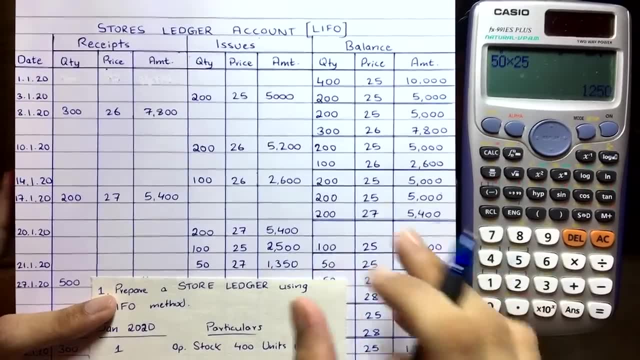 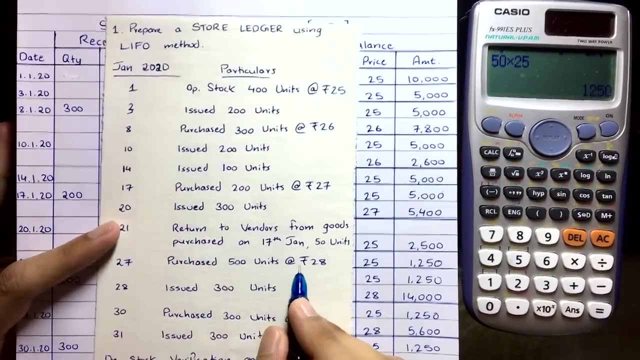 remaining at the price of what? not 27? this price? yes, so 50 into 25, that is equal to 1250. yes, that is the balance we have now understood. purchase return here. sales return here. fine, and then let's move on on 27. what is happening? purchased 500 units at the price rupees 28, so now again purchase. 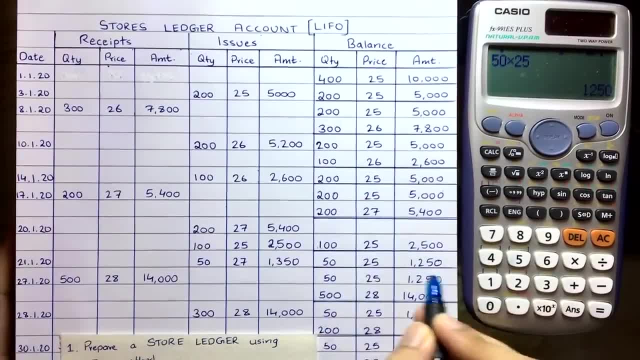 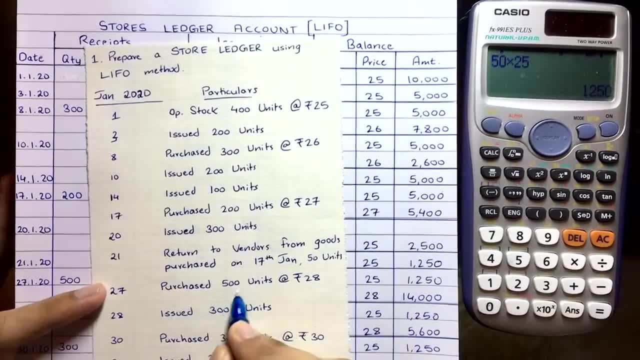 is happening: whenever we get a purchase, what we do, draw a line, whatever that is there in the balance column, take it down and then take the purchase, what we have purchased on 27th. see here 500 units at the price 28, isn't it so 500? 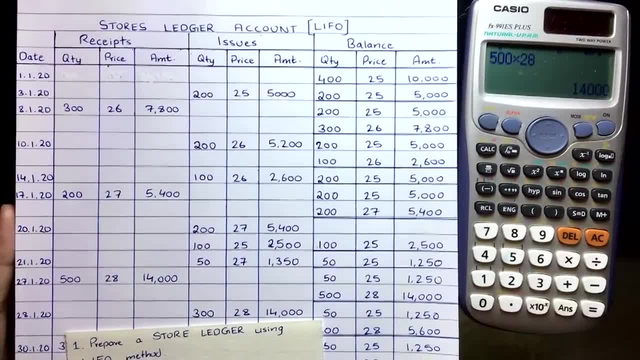 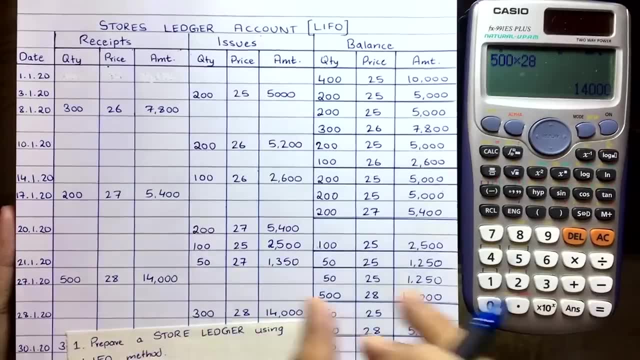 28 500 into 28, that is equal to 14 000 simple. yeah, so now what you have done: driver line took it below. and then this thing: you have to copy and paste it exactly below that: yes, so 528, 14 000 simple. yes. 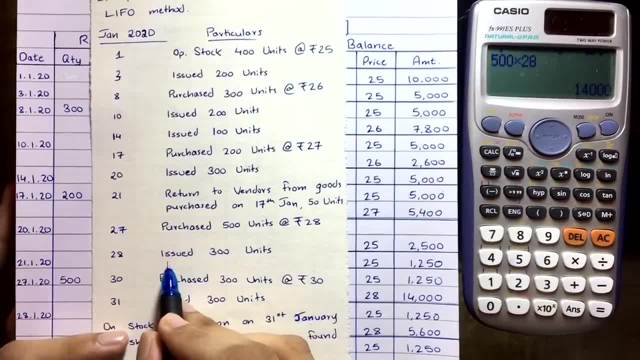 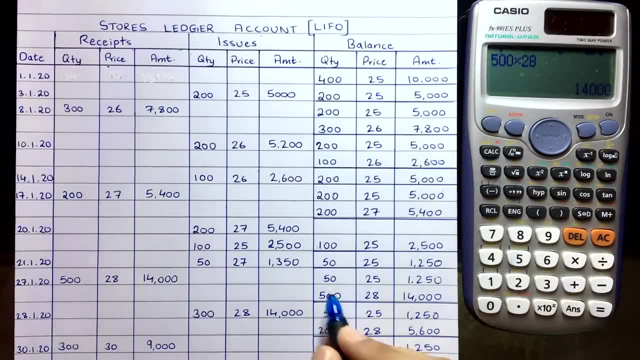 and then next 28 january- see here, 28 january, what is happening- issued 300 units. 300 units are going out of the warehouse. yes, so how are you going to do that? life form method? see here what you have here in the balance. this is the balance you have. this is what is there in the warehouse. so now you have. 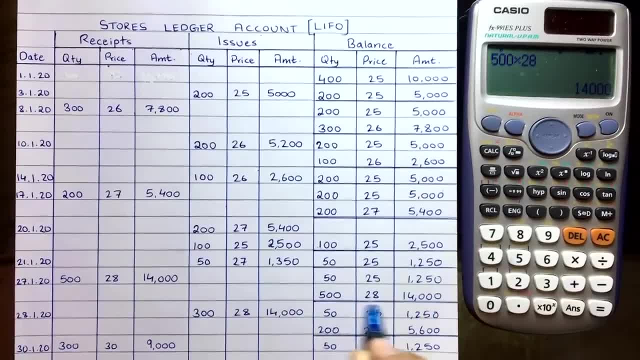 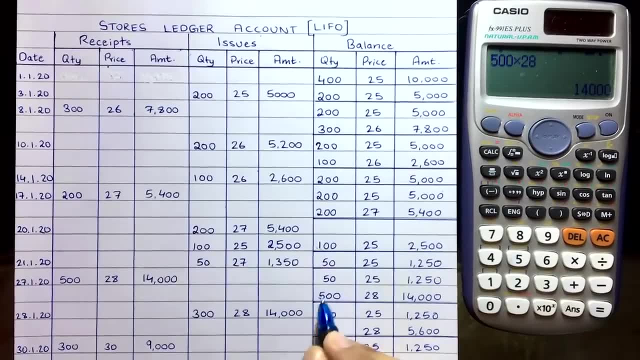 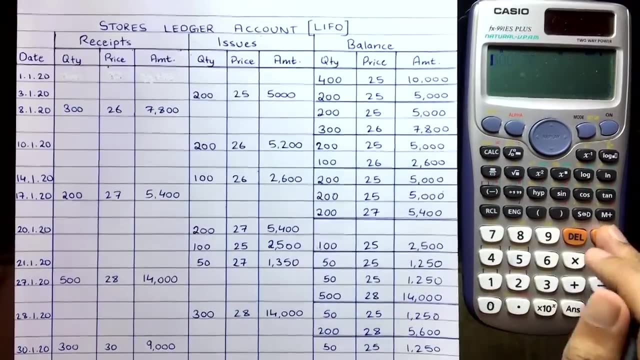 to touch the latest, the most recently purchased lot. so this is the one right. 500 one. yes, so you have to send out 300 units out of this 500. yes, see here. issued 300 units. so you have to touch the latest lot, 300 at the price 28. so see here: 300 into 28, that is equal to 8400. sorry, i have done a. 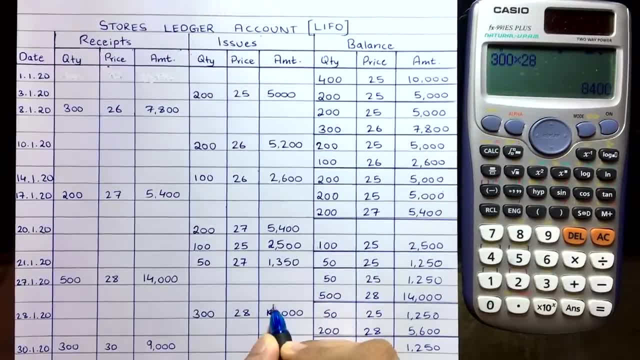 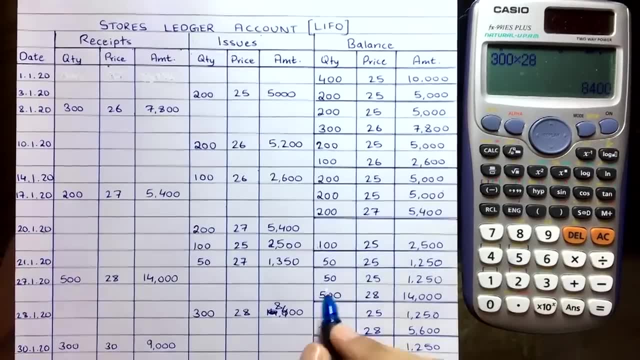 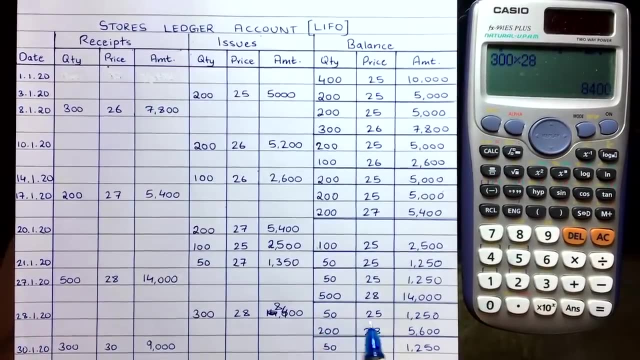 mistake over here. this is 8400, okay, 8400, right, simple, yeah. and then what you have to do: see here what is left. you have to write it at the right side, right in the balance column. so we haven't touched this 50, so 50 will be the same: 50, 25, 1, 2, 5, 0. but then here you have touched, right you. 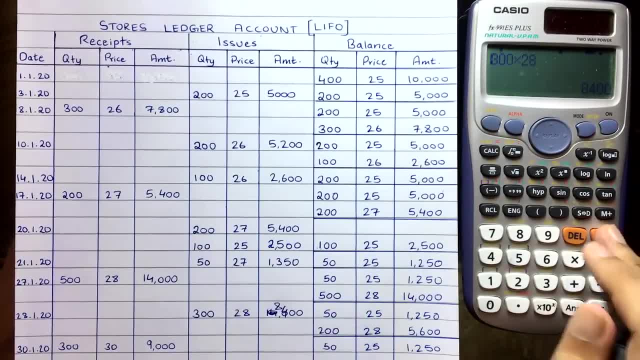 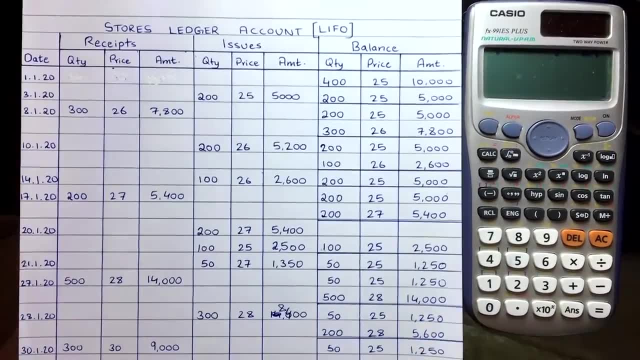 have sent out 300 from the 500, so the remaining is 200. so 200 into 28 that is equal to 5600. simple yes, okay. and then what has happened? see here: on 30th january, we have purchased another 300 units. 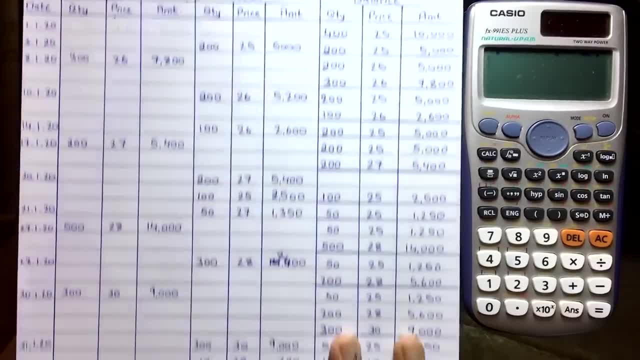 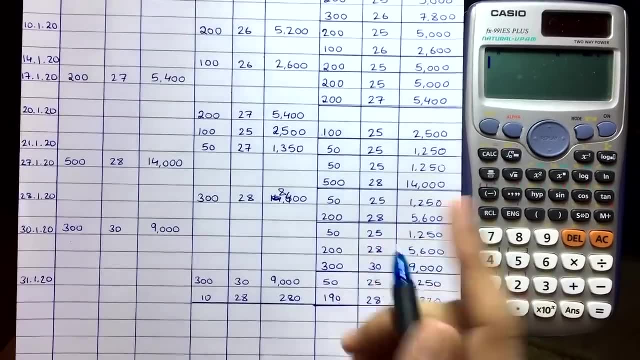 at the price: 30. so simple, it's a purchase. what we have to do whenever we purchase something simple: draw a line. yes, that's what we do. draw a line, whatever that is there in the balance column. take it exactly below yes. so see here: 50, 25, 1, 2, 5, 0. take it below 200: 28. 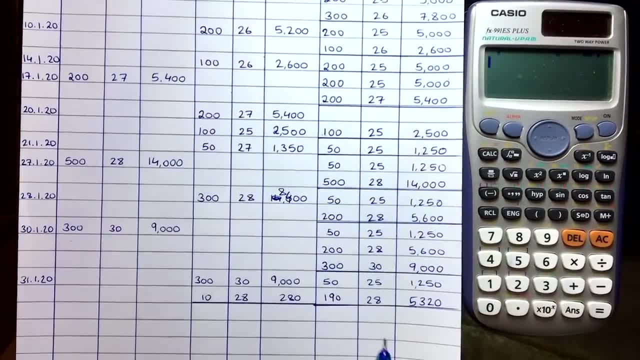 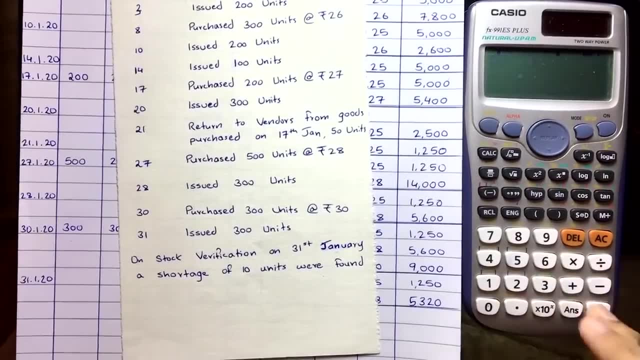 5600 was there in the balance column. take it below and then. what do you have to do? you have to see what you have purchased. you have purchased 300 units at the price rupees 30, so 300 into 30, that is equal to 9000. cost: yes, 339 000, simple. so this is what you have purchased on 30th january. 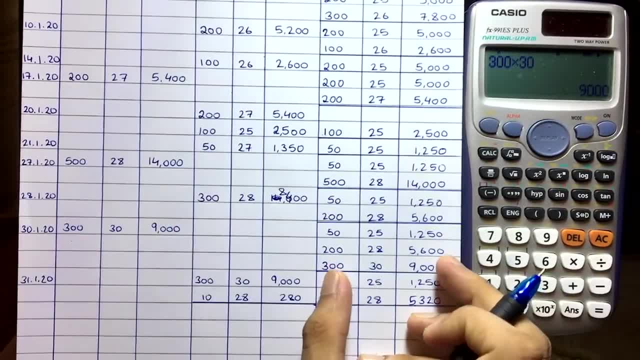 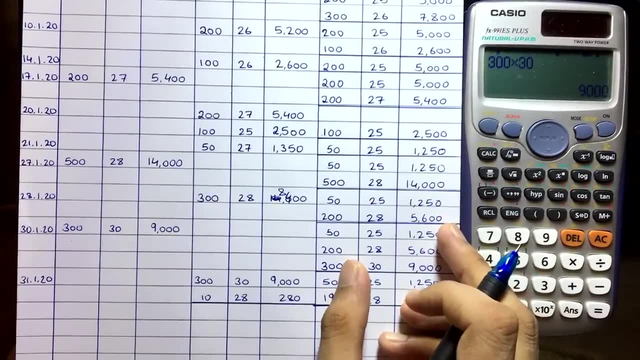 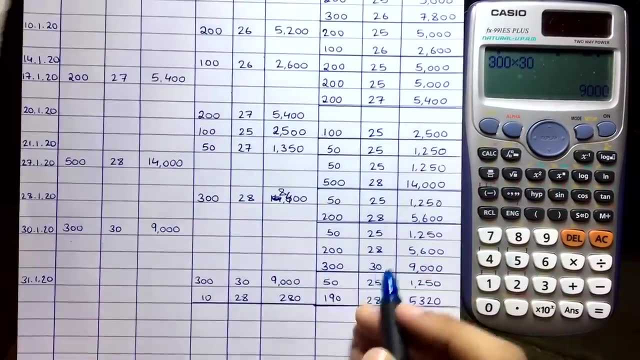 and then you have to take this and copy that exactly below: yes, 339 000, simple. so now this is what you have in your warehouse: yes, and then what has happened? let's see: on 30th january, we have first issued 300 units. we have to send out how much? 300 units? simple, let's do that. so here see. 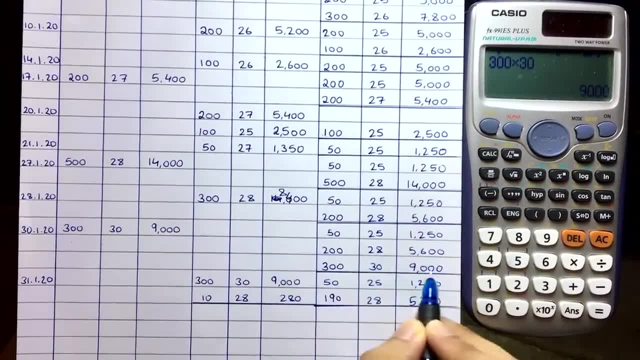 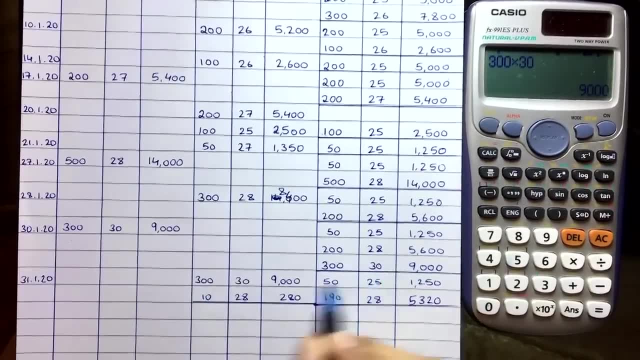 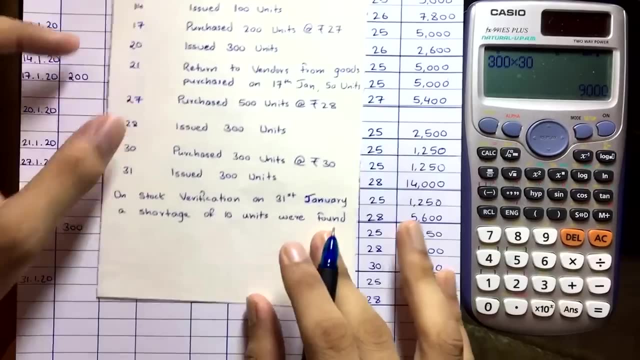 how much? 300 units. so you have to use the latest lot, yes, lifo method. so the latest, last in, first out. so you have to touch this 300 lot, so 339 000. so this issue is made right simple. yes, so now it's almost done, but at last we have said a statement- see here on stock verification. on 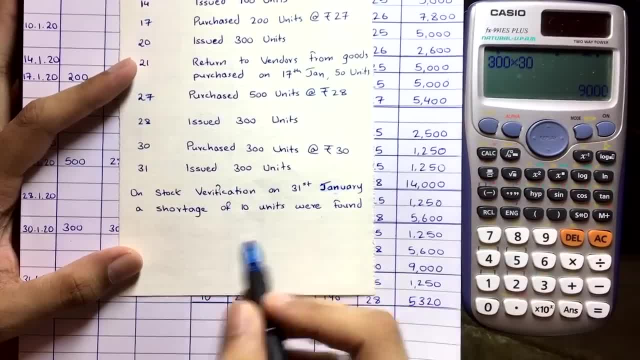 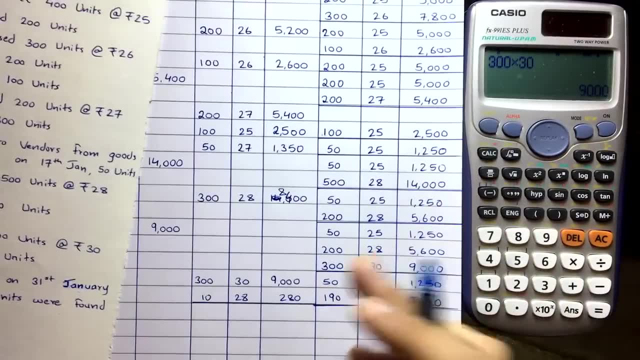 31st january, a shortage of 10 units were found. shortage means what? shortage means? it is no longer there in our warehouse. so simple thing: if it's not there in our warehouse, you have to send it out, okay. so shortage will always come. on the issue. 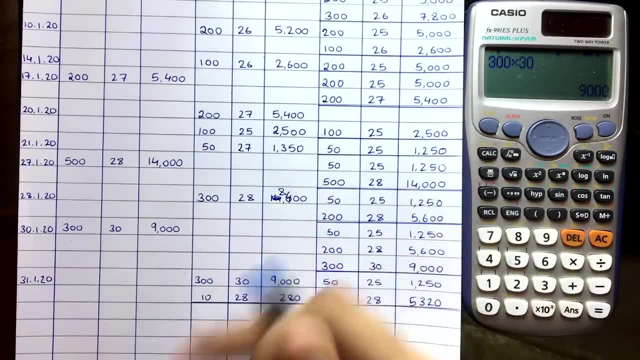 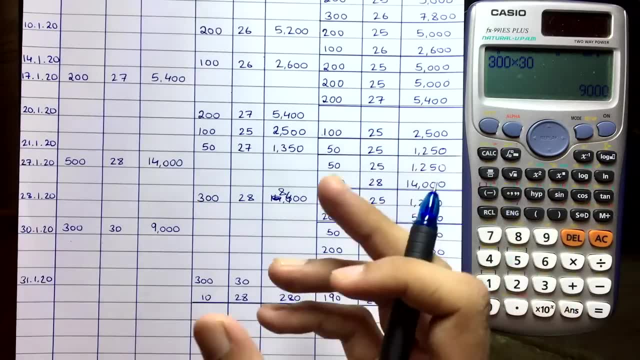 side, it has gone out of the warehouse, we don't have it. okay, if it's a surplus, let's say we have, you know, surplus. we have found some units extra. yeah, it was lost before then we found it. then what we have to do, that surplus has to taken on the receipt side, because we are getting something. 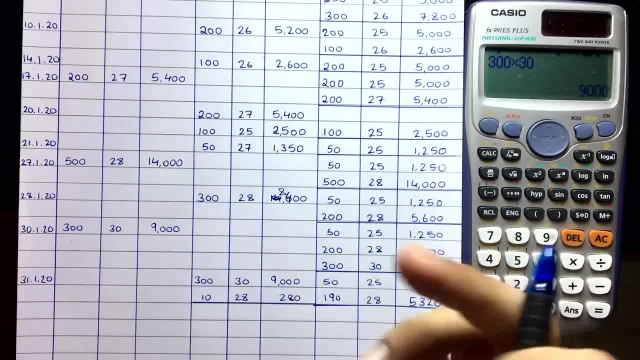 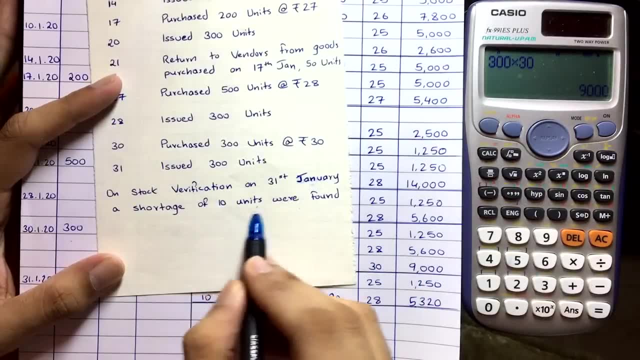 extra now, so that extra has to come over here and if there is any shortage, it will come over here. so it's very simple as that. yeah, so treat the shortage as issues, okay. so see here, 10 units were found. yeah, shortage, it's not found. like shortage was found. yeah, we have lost it. it's an abnormal. 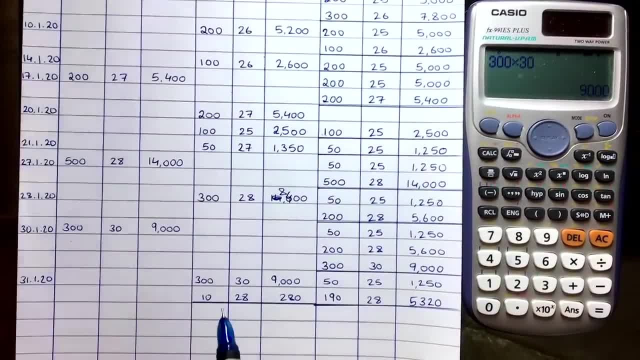 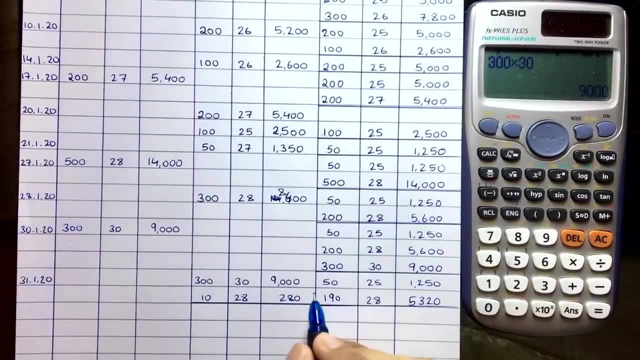 loss understood. so if it's a shortage, then what you have to do it's a deficiency. it's a simple thing: throw it out of the warehouse. think like you have thrown it out of the warehouse and make an issue: yeah, so see what we had. so i've directly made the issue here, only so. it's very simple, see. 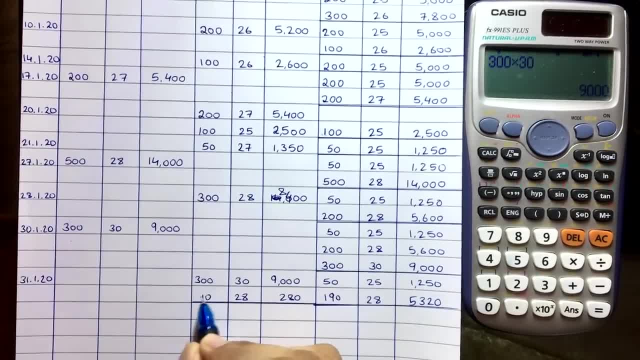 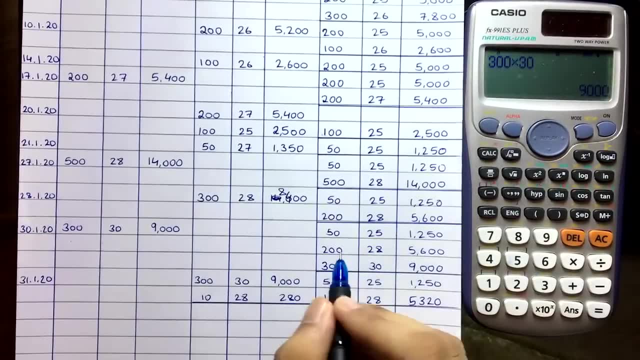 here directly. i have taken 10, we have lost 10 units. we have lost 10 units. we have lost 10 units at the price 28. so now this lot is gone, right? 300 lot. so we have to touch this lot, okay, 200 lot. 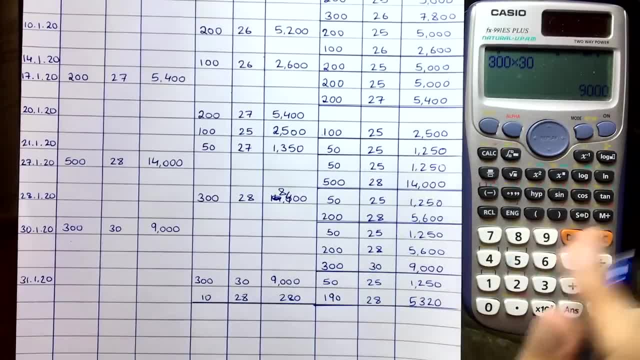 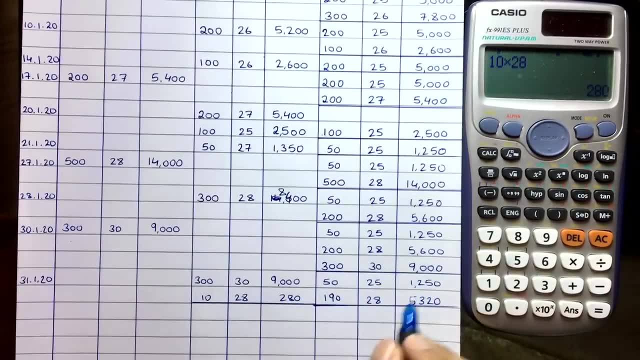 so from here, 10 units are gone. let's assume like that: yeah, 28, so 10 into 28, that is equal to 280. yes, so this is what is going out. so now what is remaining? you have to take it here, so we haven't. 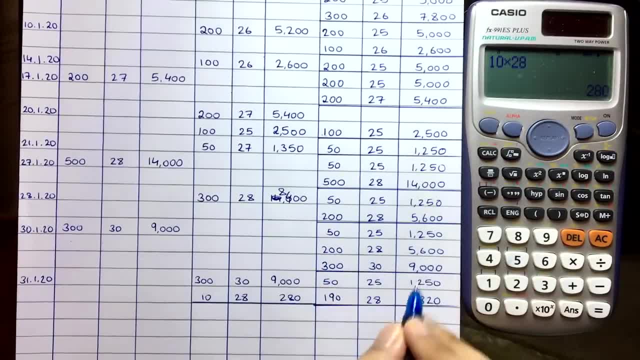 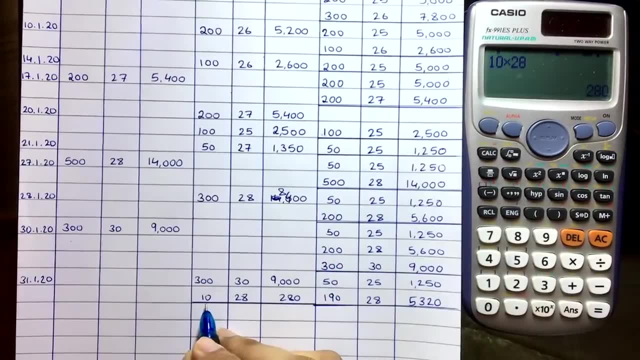 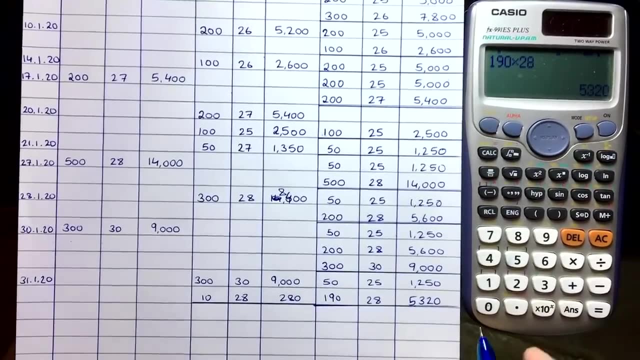 touched this 50 lot, right? so 50, 25, one, two, five, zero, exactly. you have to write, and then 300 is completely gone. so ignore that. and then here 200. from this 200 we have thrown out 10, so remaining is 190. so 190 into 28, that is equal to 5320. simple as that. yes, this is what is left in. 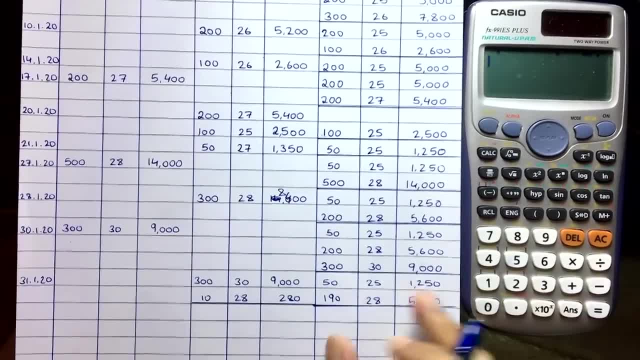 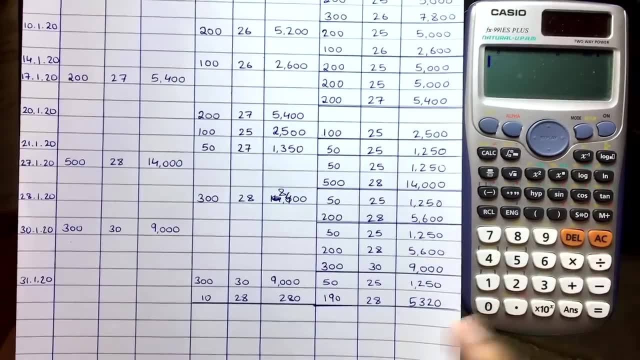 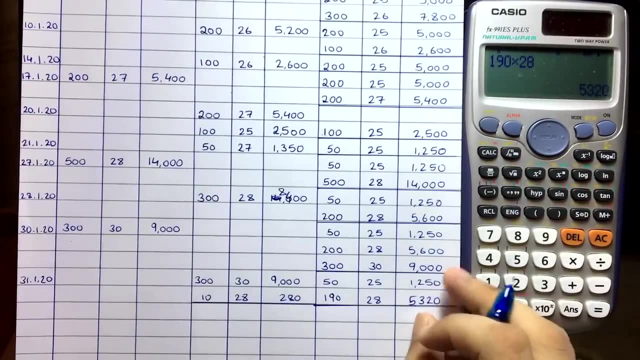 the warehouse and this is your closing stock. okay, you have to add this and do the closing stock. how will you do that? 50 into 25? yeah, that is equal to one, two, five zero. and then this thing: what is that? 190 into 28? that is five, three, two zero. yes. so now, if you add these two together, one, two, five, zero. 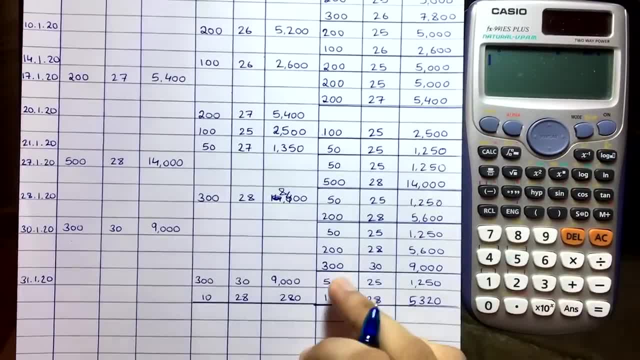 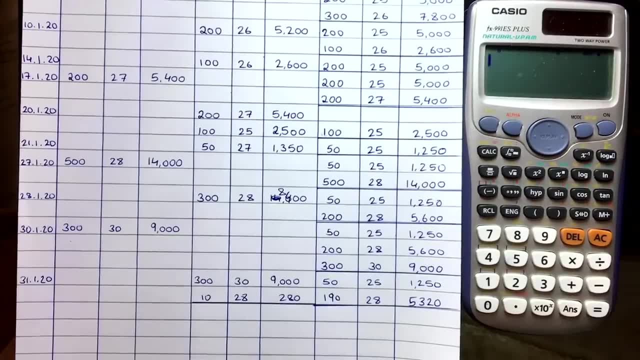 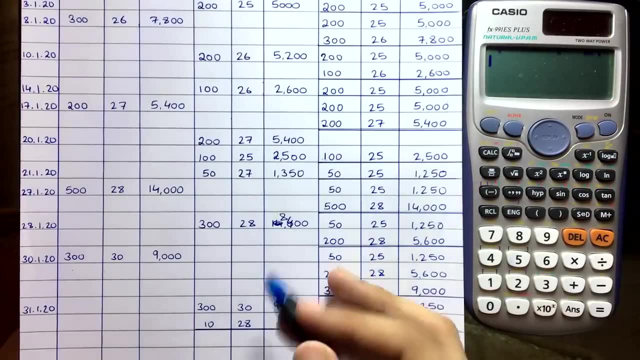 plus five, three, two, zero: this is the value of your closing stock and this is the quantity of your closing stock. 50 plus 190, this is the quantity of your closing stock. simple. so this is what is lifo. it's very simple. whatever that has come in last, you have to throw that out. okay, so you have to do exactly opposite. 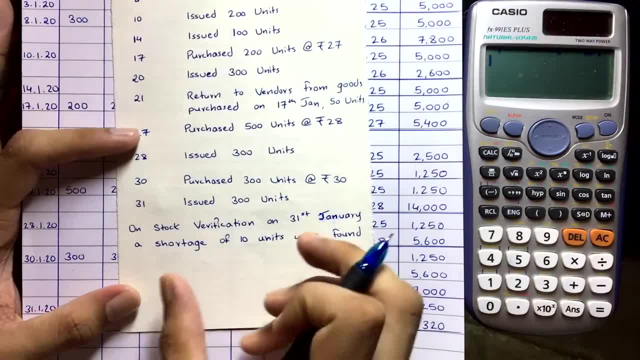 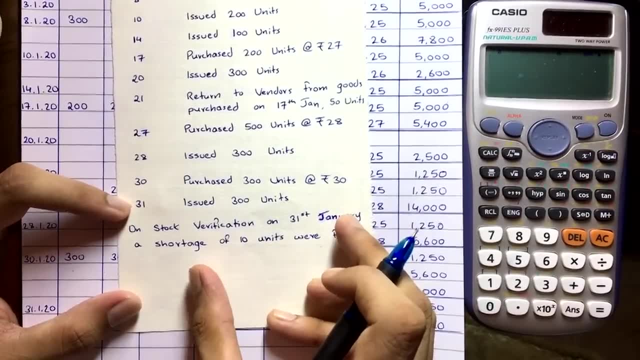 of fifo. it's nothing, but here you have to be very careful, okay. so see here: stock verification. here it was given 31 january at last, but sometime, what can happen? this statement will be given at last, okay, but the date will be the date of somewhere here. 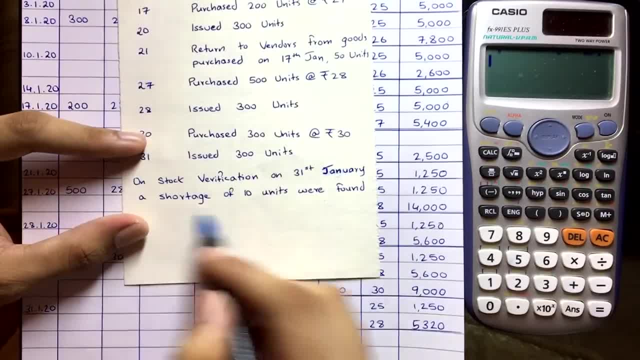 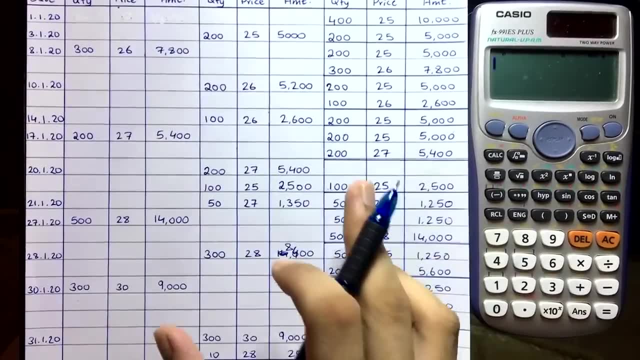 let's say, 10 january, 11 january, and what you will do if you came to know about this at last? then you can't make an entry directly here somewhere, right? yes, you can't do that. the entire problem would be wrong, the entire solution will be wrong. so that is why read the question.